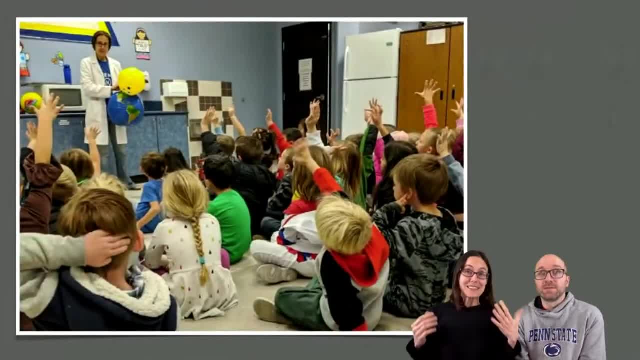 really fun giveaway items. So Science Mom all started because I volunteered to bring science experiments to my son's second grade class And my name changed From science Andrew's mom to science mom, And it stuck For about five years. I traveled and 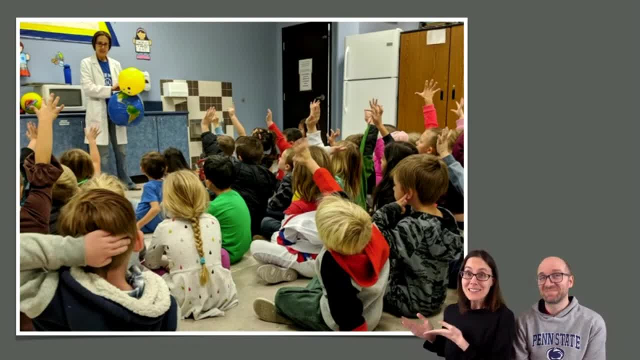 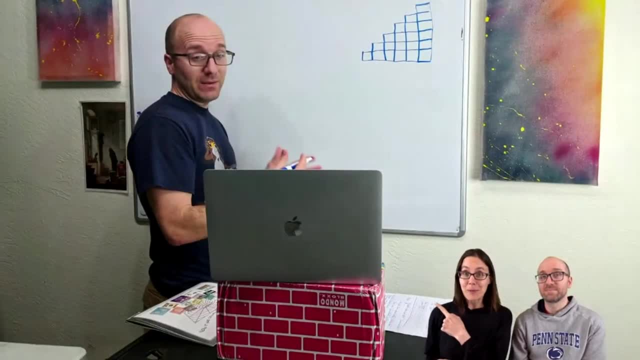 visited more than a thousand elementary school classrooms in the Las Vegas area doing science demonstrations And I loved it. And then, when the pandemic started, we had a laptop and we had a cardboard box And we decided that was enough for us to do free math and science lessons for people. 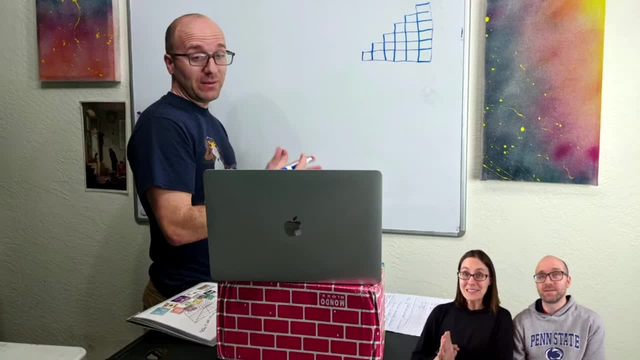 who were stuck at home during quarantine And we did a series called Quarantine And I roped in with my dad, who is a mathematician. That's right, 52 fun lessons of us and the world trying to figure out how do we handle a quarantine like this. 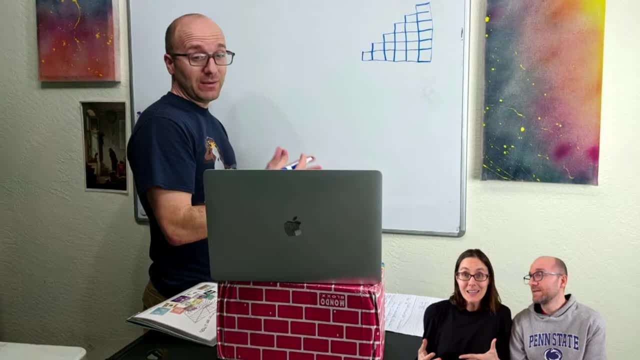 Math Dad got his name because when I would do science demonstrations in the Las Vegas area, I would introduce myself. I would say I'm Science Mom And then invariably I would get a couple of kids who would say: if you're Science Mom, 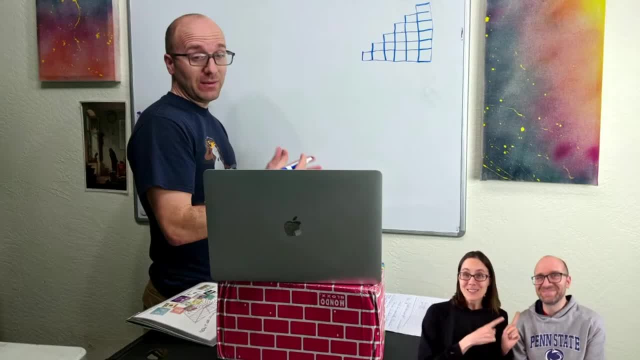 where's Science Dad? And since Serge has a PhD in mathematics, I said: you know, we really should call him Math Dad because he's a mathematician. So that's how that works. That's how that all started. A couple more quick hellos. Hello to Manny watching in Chicago. 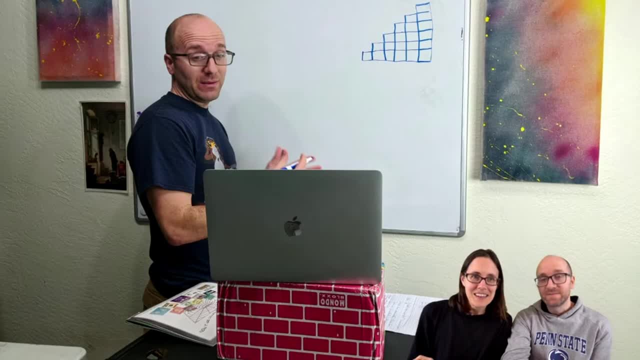 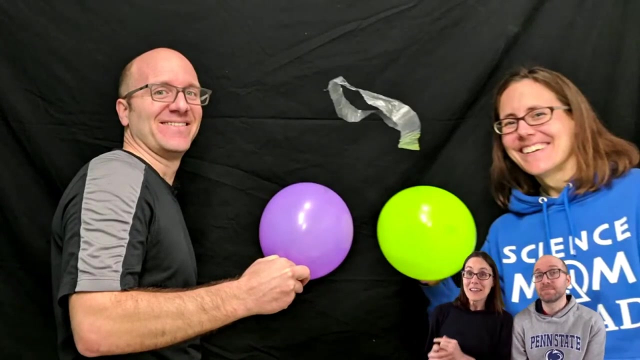 I see the EC family watching from Massachusetts. Annika Elizabeth from Georgetown, Texas. Good to see you all here. Texas, Ontario, Chicago, Excellent Canada. I'm loving this. One more quick story to round out our introduction: Doing these 52 math and science lessons for quarantine. 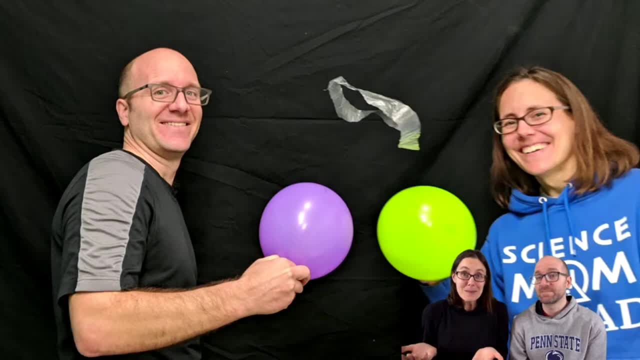 we really enjoyed working together And I thought you know what. I want to keep doing this. So we made a chemistry course and then an earth science course. And then I said: Math Dad, you teaching college full time and us doing these classes is too much. One of us has to quit their job. 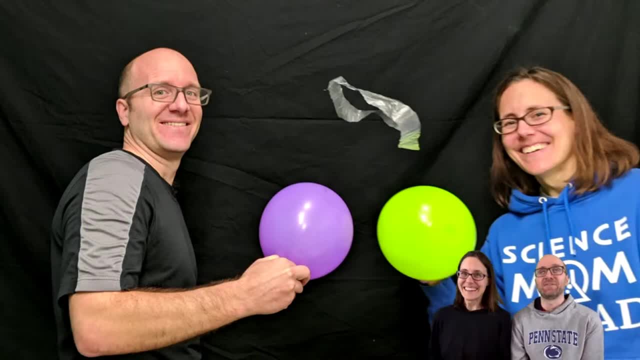 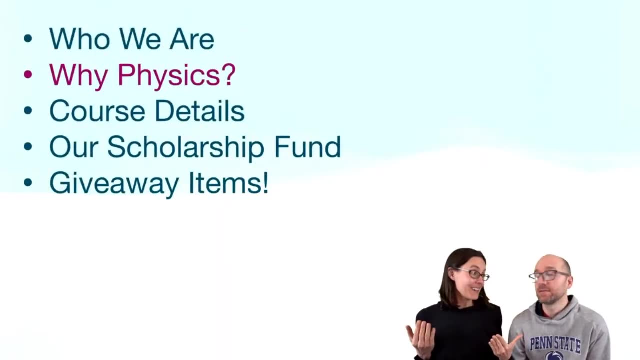 And he said: OK, That's right, I loved my job, but Science Mom managed to steal me away. Yeah, And so now we live in Virginia. And why should you study physics? Because physics is awesome. Physics is awesome, So not only when you study physics. 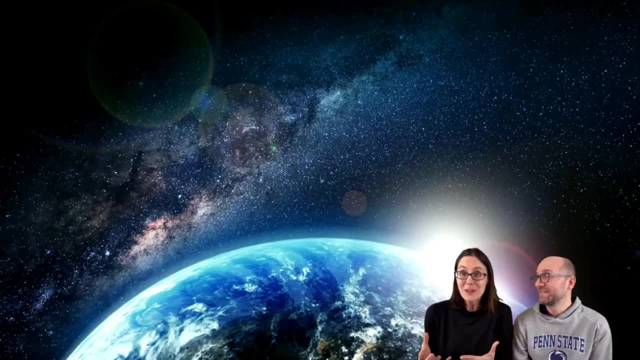 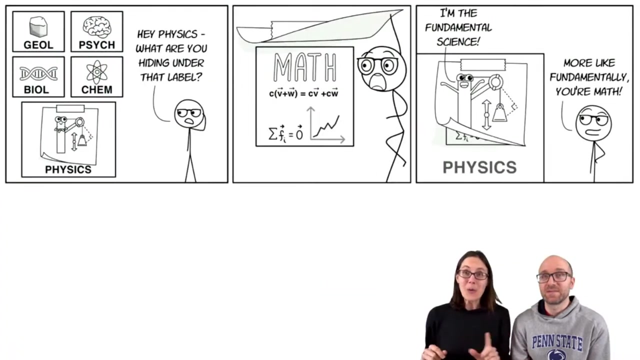 not only do you increase your critical reasoning and your ability to solve problems, but physics is the foundational science. If you have a good understanding of physics, then you will better understand every single other branch of science. And it's just awesome. In our physics class we are going to start: Oh, why should you study physics with us? 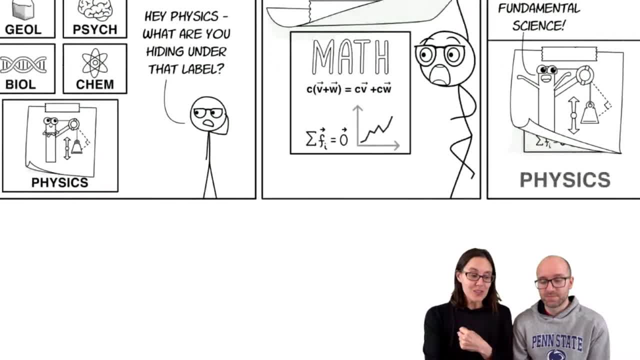 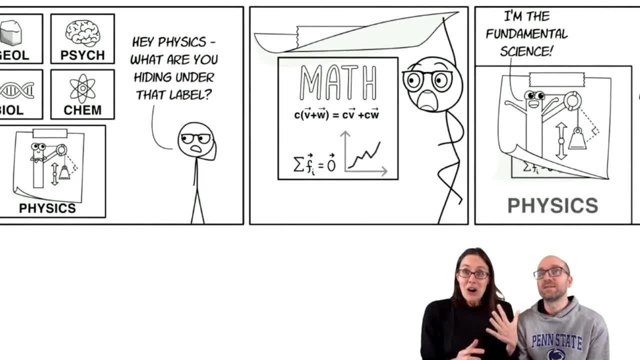 I made a comic about this. It's in our notes. So if you look at geology, psychology, biology and chemistry, He's like, hey, physics, what are you hiding under that label? And then he lifts the label up and says it's math. 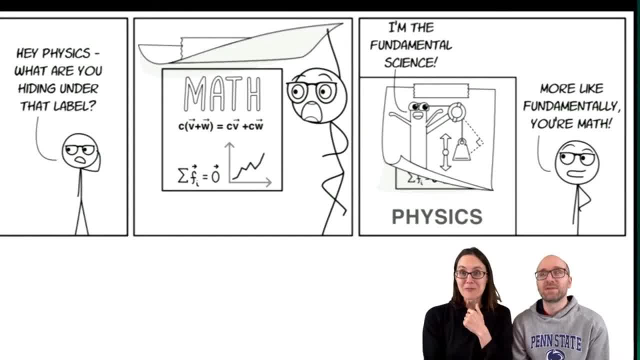 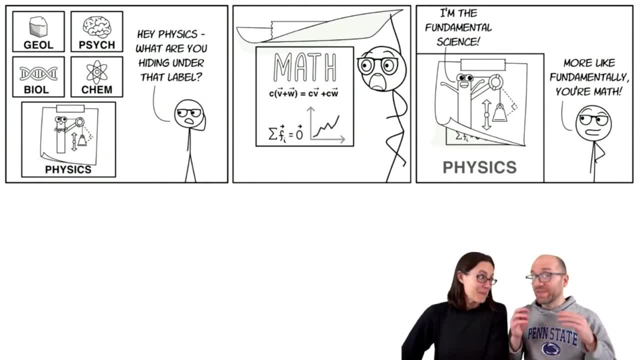 And physics says I'm the fundamental science And he's like more like fundamentally your math, And there's a lot of truth to that. Physics is very quantifiable And you can come up with exact answers in a way that you can't in many of the other sciences. 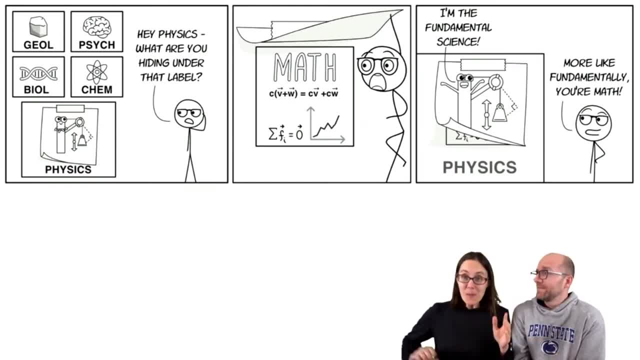 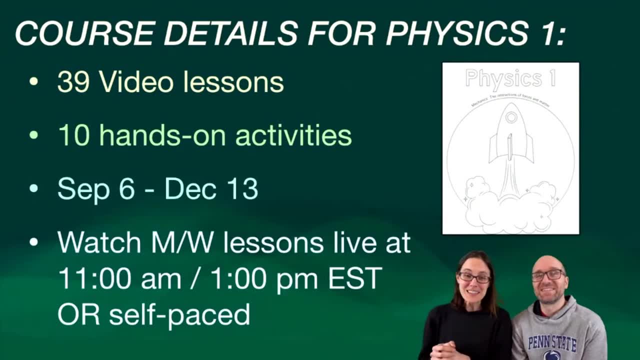 And so science mom plus math dad equals the best physics class for middle schoolers ever. That's why you should take physics with us- And here are some details about our course. And math dad. will you put the link to our giveaway in the chat? 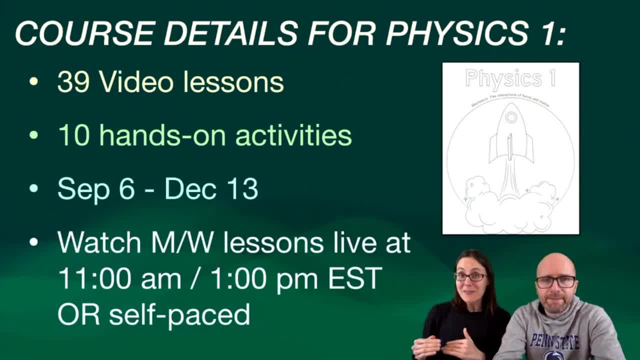 We're sharing a link where you can enter for our giveaway. We're going to do it live And then we'll take questions about our course, But I wanted to give a quick overview before we did that. So we have 39 video lessons in our course. 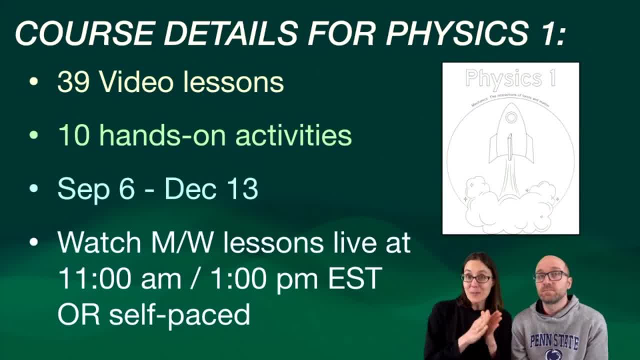 There are 10 hands-on activities. It's going to start September 6, 2023 and run through December, And there are three lessons a week: The Monday, Wednesday lesson, And then the Sunday lesson, And then we're going to have a little bit of a live session. 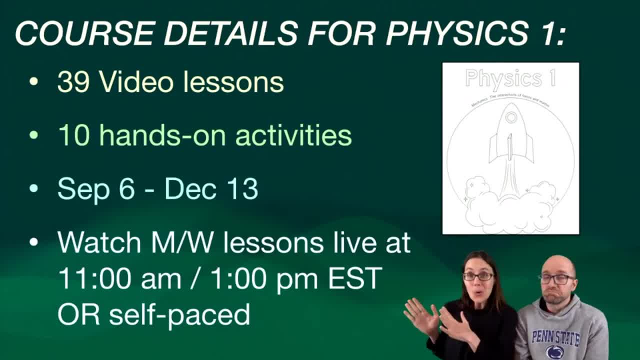 So you're going to have to do a little bit of a live session, But if you aren't available at these times, that's totally okay, Because they're all recorded. You can watch them at any time. That's right, And you don't have to attend any of the live sessions. 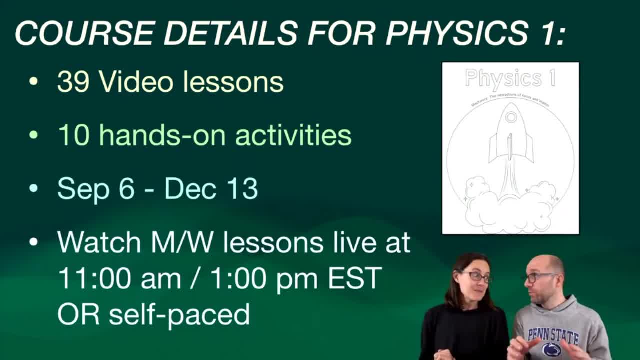 If you just want to complete the course on your own time, all the recordings will be there. You can even participate in the polls after the lessons are done. That's right, And we're calling it physics one, because this course in fall is going to cover mechanics. 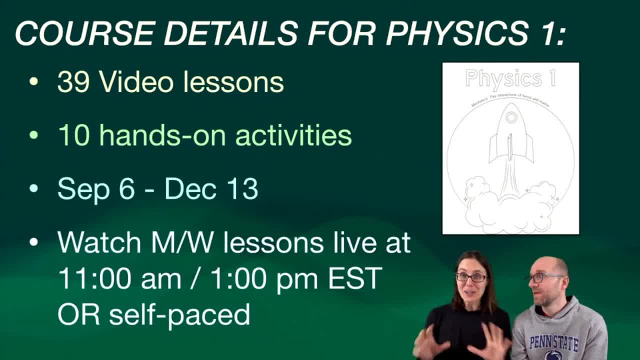 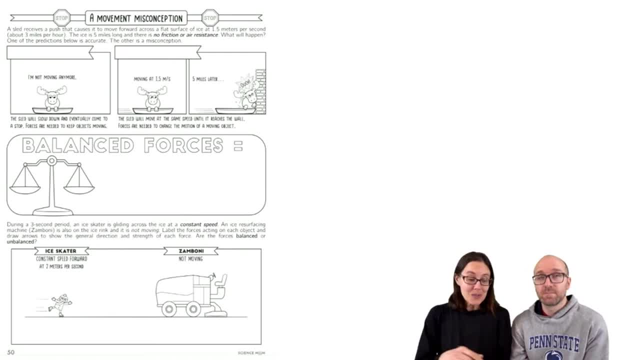 And then in the spring we will have physics two, which will cover electromagnetism, sound, light waves and all of that. Now, I love drawing and I love cartoons, So I make doodle notes that go along with each lesson. 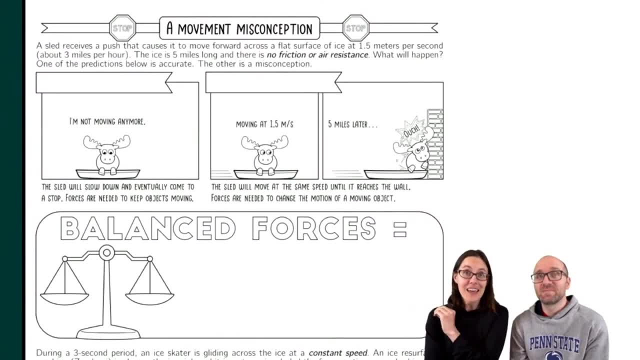 So every single lesson will have a note page, something like this, And there will be parts during the lesson where we'll pause or we'll model. You know we'll be filling out the note page And this is one of the things that we consistently get a lot of feedback with our classes like earth science and biology. 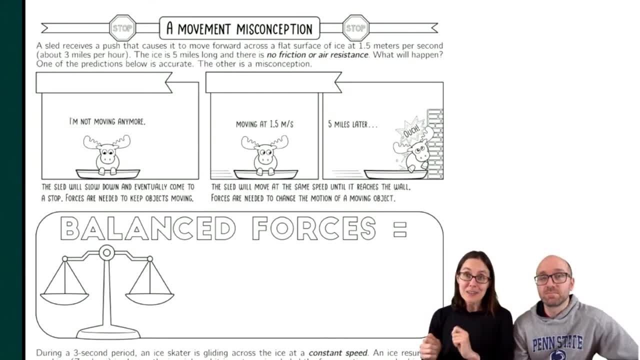 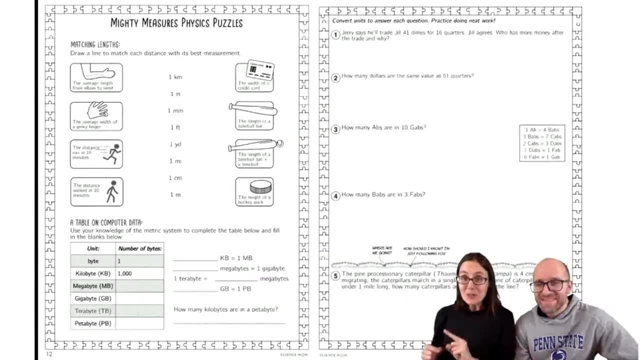 that people really love this style of notes and how interactive it is and how it helps the student to learn more. So each lesson has note pages and each lesson also has physics puzzles, because physics, like we said earlier, it is very quantifiable. 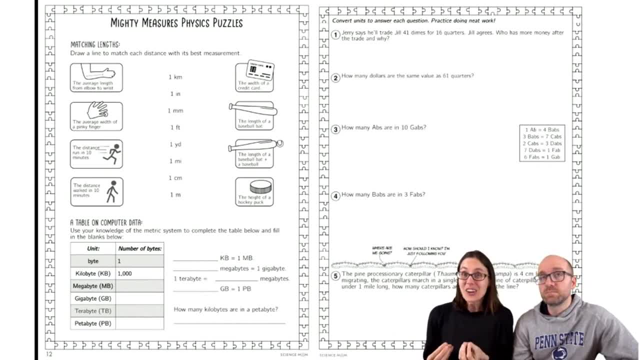 There's a lot of math and physics And if you don't do practice it, you're not going to learn as deeply. So every single lesson does have a couple of pages of physics puzzles, So students can can really get their hands into the material and make sure that they're understanding it. 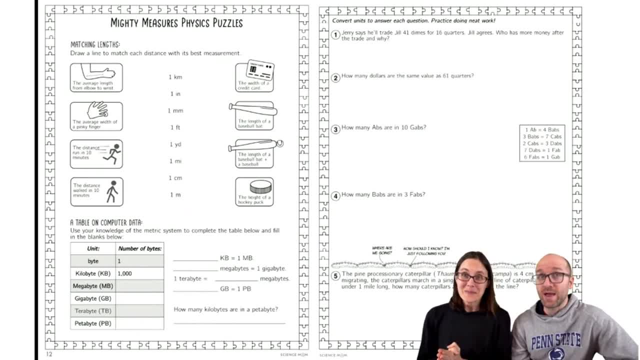 That's right. It's the only way to learn it. You actually have to do the calculations, You have to Mm-hmm, Do the thinking and get your hands dirty. That's right. And hello to everyone watching in Canada, to Eugenia, to Charlotte, to Elena. 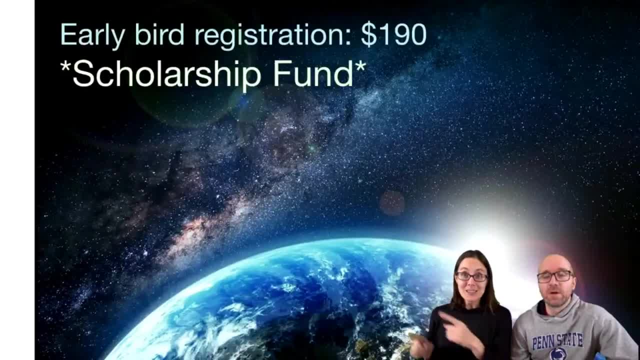 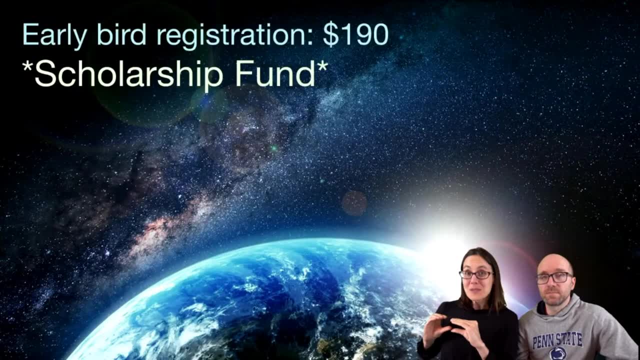 It is good to see you all here. We are ready now to give a shout out to our scholarship fund. We have patrons on Patreon And there's a scholarship tier where certain patrons will support scholarships every month. So on our website we have a scholarship form. 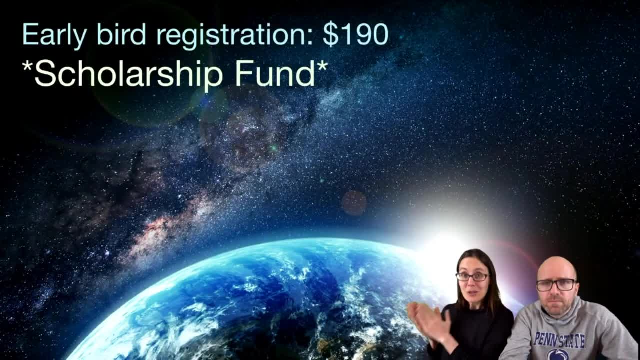 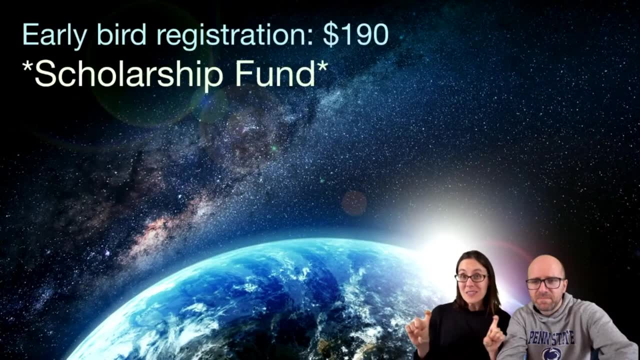 Every month we give away scholarships, But for physics we're doing a special early bird registration to promote our scholarship fund. Math data will put the link to that in the chat as well. It's also in the description. We're going to award those scholarships on April 15th. 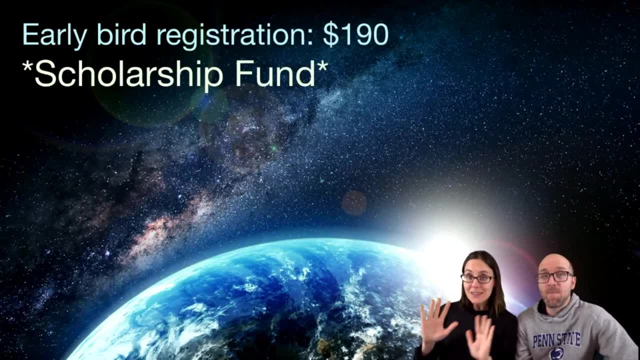 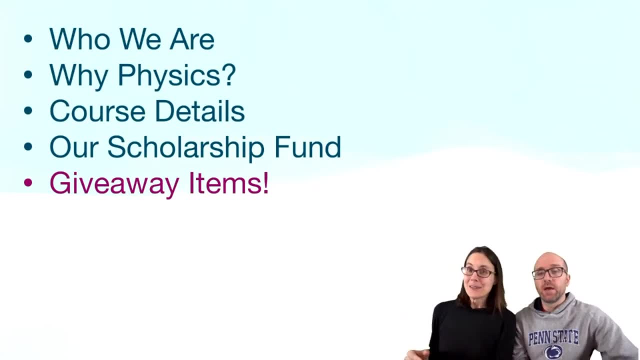 That's one that will close five days from now. Five days. There are five days left to enter for a scholarship for physics. And guess what we're at now? The giveaway items, Our giveaway items. Well, let's, should we ask if there are any questions and give people sufficient time? 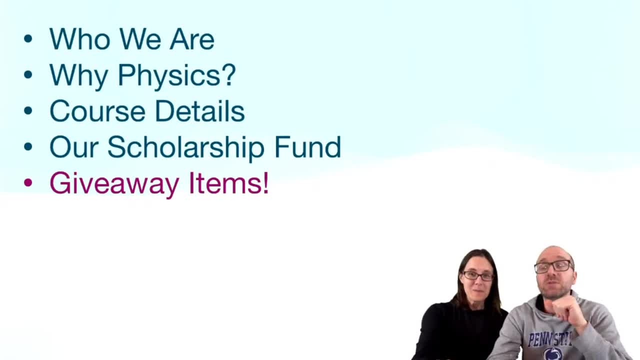 So OK, Emily's asking: can you buy the year long program Or is it two separate purchases? We don't have it set up yet. Eventually we'll figure out how to do it, but we'd have to actually create the second half at the moment. 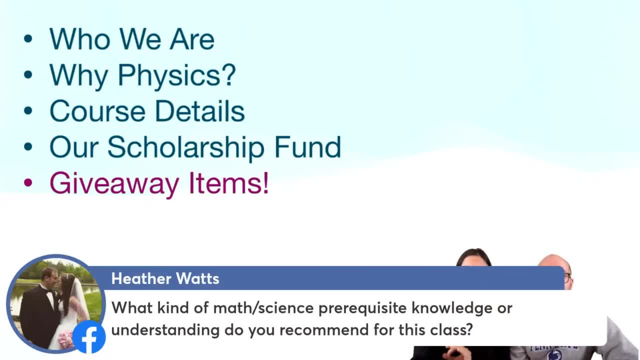 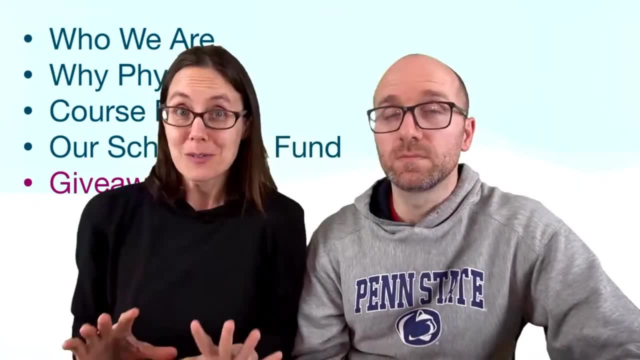 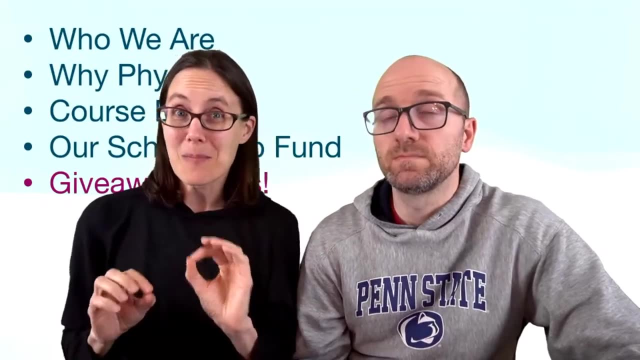 It's not possible. And great question from Heather: What kind of math and science prerequisites are do you recommend for this class? We want to make it really accessible to a middle school audience, And so we're keeping the math level fairly basic. You don't have to have algebra, but you should have a basic understanding of 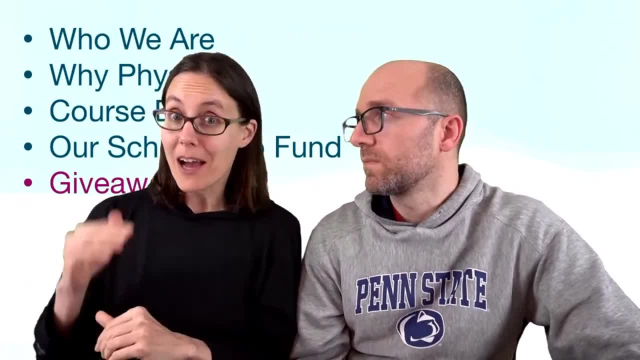 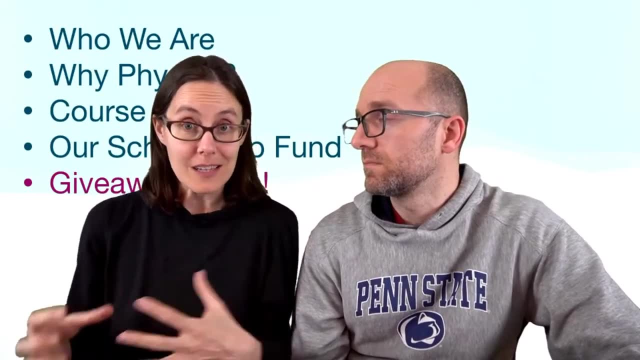 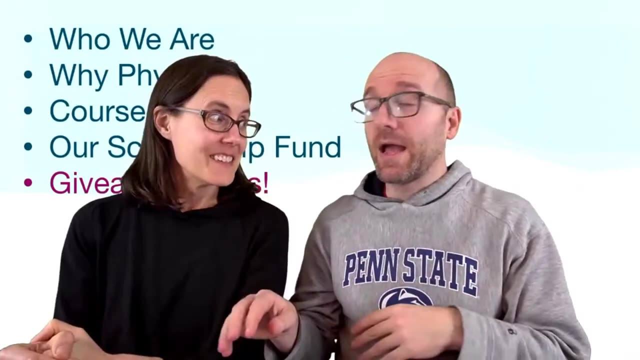 the math variables and on page six in the notes preview, We have a list of just some basic skills: understanding what a variable is, being able to, being strong with fractions and decimals in addition and subtraction, basic arithmetic. just being fearless, I mean if numbers cause you to run and hide or if they're unpleasant to deal. 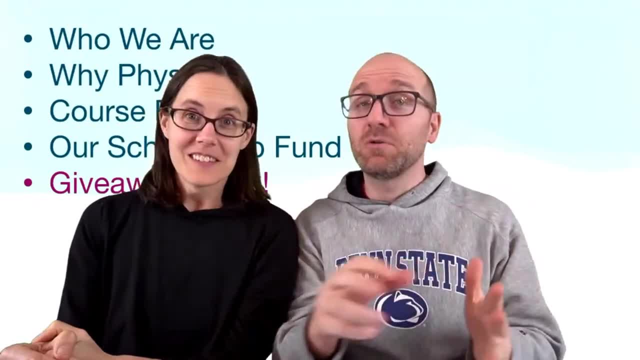 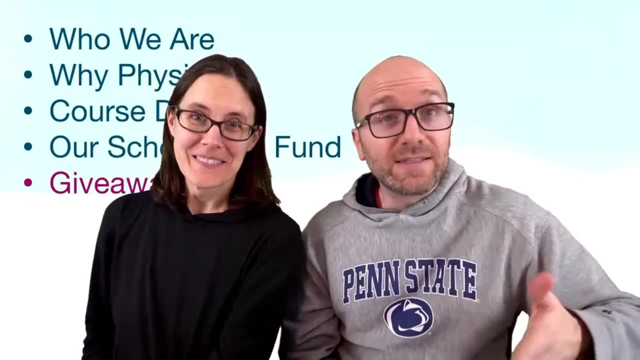 with you might not enjoy the physics class because numbers are going to be all over the place and you can do numbers We will make you absolutely can join us for physics. That's going to be awesome. So if you've had our grade six math course, for example, you'll be totally ready. 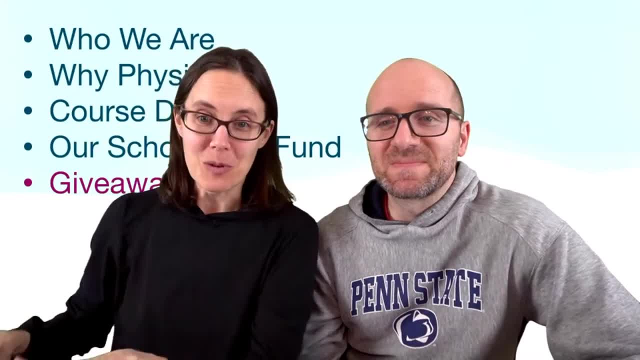 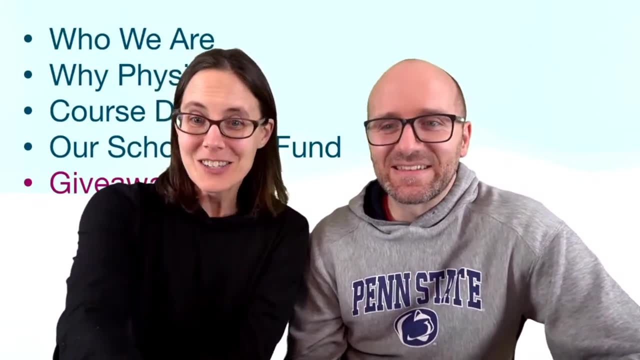 Totally ready Answer. just a couple more questions and then we'll do our, our giveaways. Oh, Hannah says our boys are doing biology right now and they're loving it. I'm so glad, So glad. Trina is all registered and excited And oh good. question from Corey. 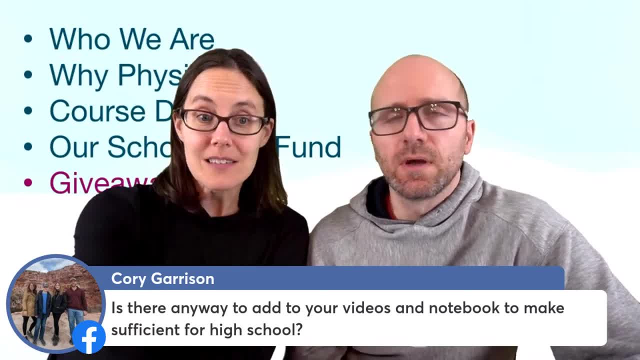 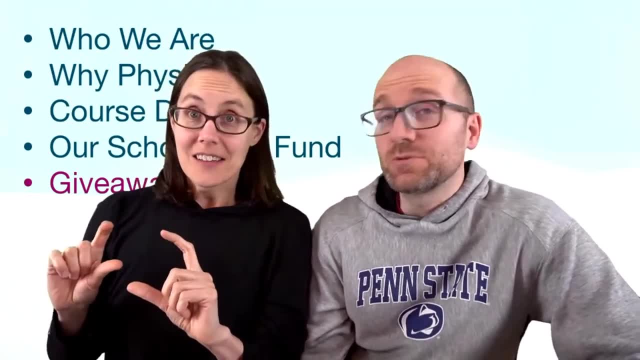 Is there any way to add your videos to notebook and make it sufficient for high school? So I would say what we're doing is going to be a substantial part of a high school physics course is. the concepts are all pretty similar to what you get in high school, but in high school there will be more math. 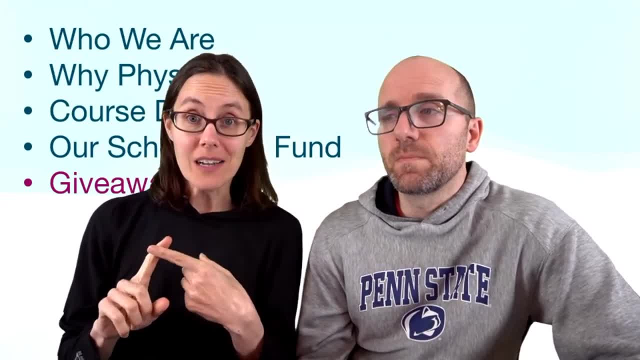 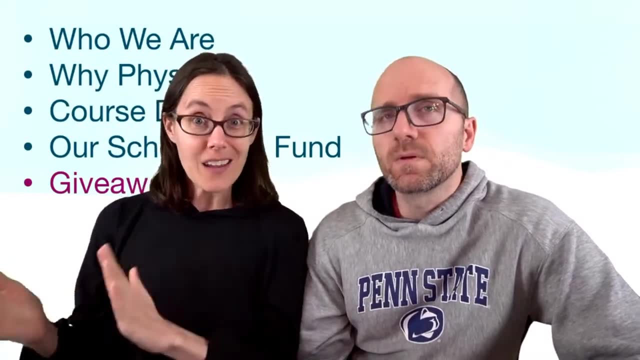 So I do have a couple of books. Conceptual physics is a really great one, And then there's a high school math book that I have upstairs. I'll add it to the description after we finish, But yes, by adding a book that has more. 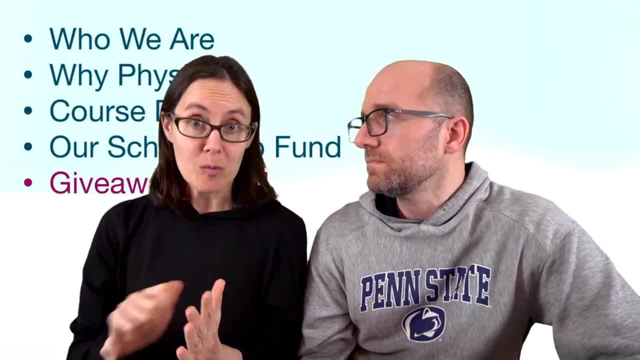 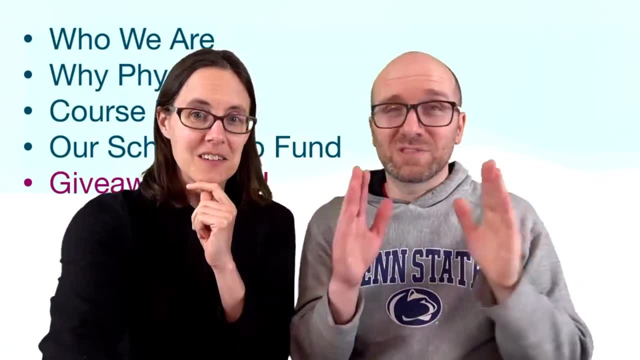 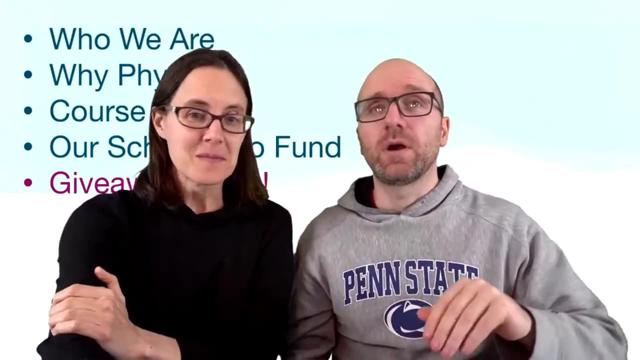 quantitative problems so that they get the practice with the algebra based based physics problems. you could adjust it for high school. Yeah, high schools have a tendency to have special requirements, though they really want to make sure you've hit all the items on the checklist and each state is different in their requirements. 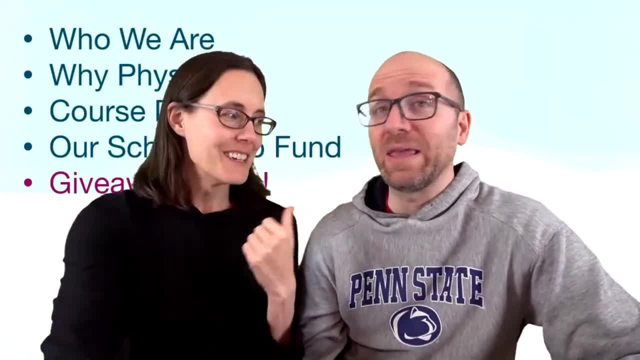 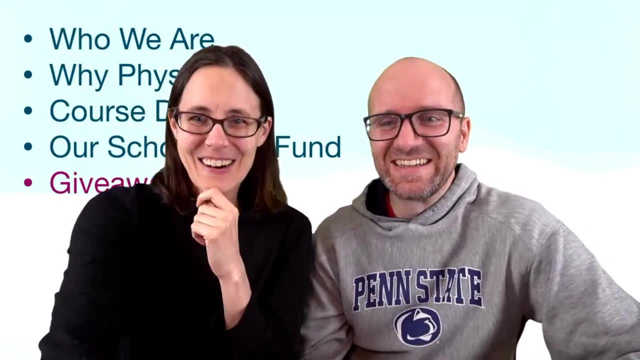 So it'd be kind of difficult to get a full AP. That doesn't want you to blame us if it doesn't work as a high school course. That's what he's saying. And oh, I saw a good question now: What age is it best for? 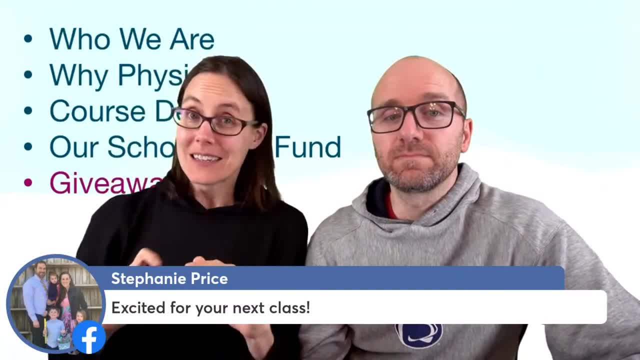 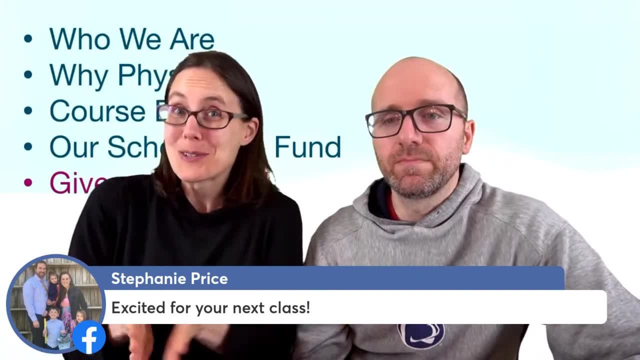 Kelly asked: what age is it best for middle school? So I would say sixth, seventh grade ish, But really we have students that are younger and students that are older. You know your student best. So I'd say if they're in middle school, chances are it's an excellent fit. 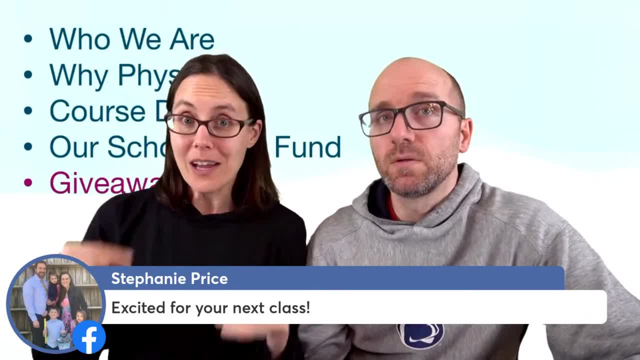 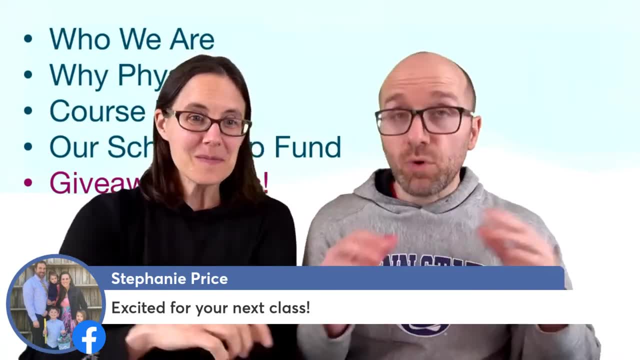 But if they're a little younger or a little older, take a look at our notes and what we have outlined And I do think we'll get some high school students in here that will enjoy it and do well, especially if they want to prep before their AP physics class. 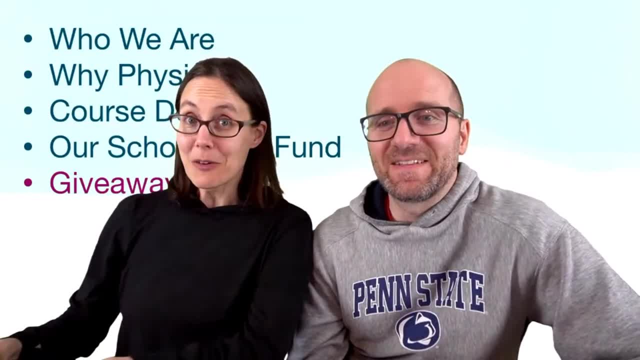 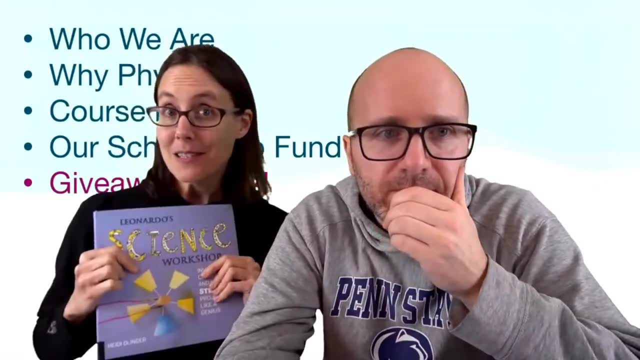 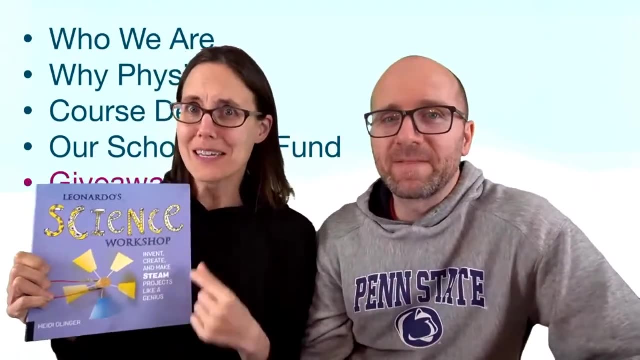 It would be a good fit. OK, I want to do our giveaway items real quick, And Math Dad, we paste the link really quick one more time. So we are giving away three of my favorite physics books for middle school students, And the first one, Leonardo's Science Workshop, has really nice hands on. 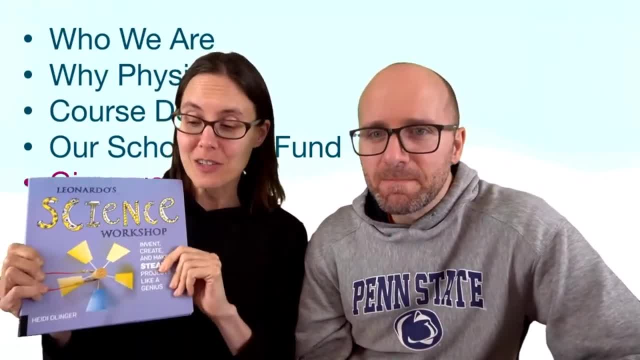 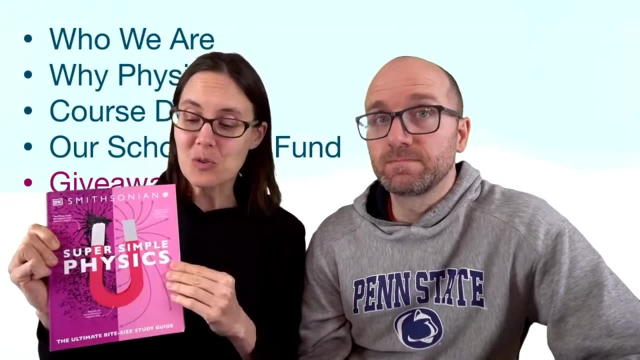 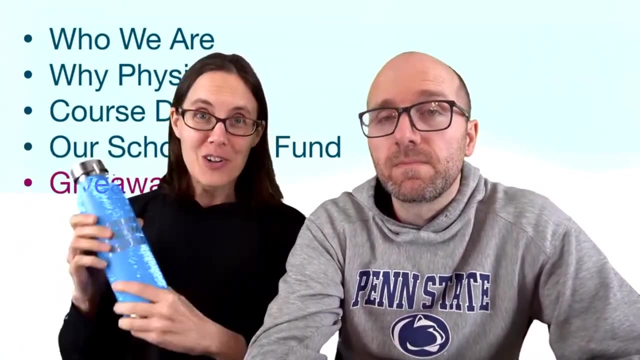 activities, but also does a great job of just weaving in a storyline of Leonardo Da Vinci. I really like the Smithsonian's super simple physics books. It's got great material, lots of cool illustrations as well, And then projectile science. So this bundle of books plus a water bottle and as much as many stickers and fun. 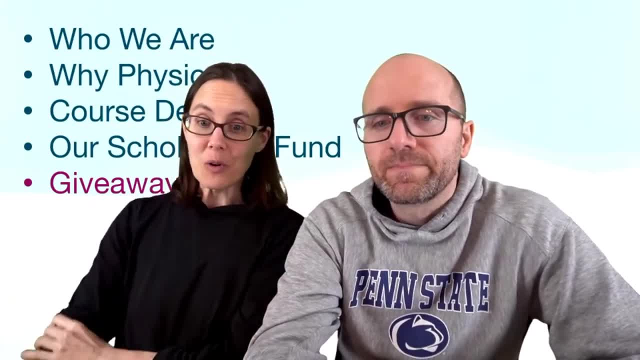 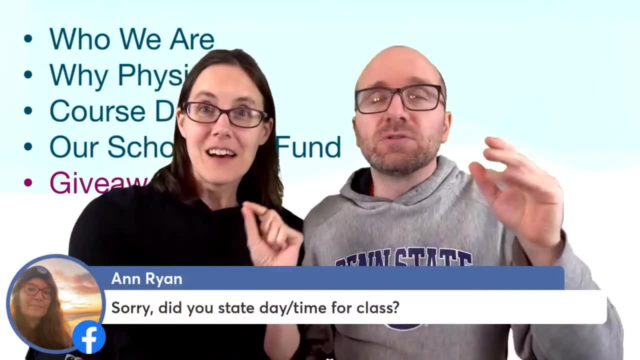 goodies as we can fit into a medium flat rate box is the first item that we're going to give away. So Emily asked no. somebody asked for the time again. The time will be 11 am Eastern and 1 pm. 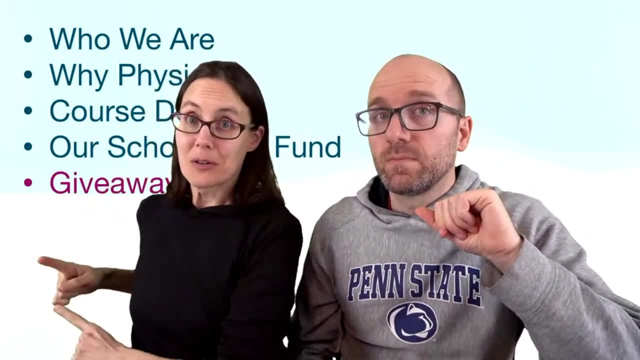 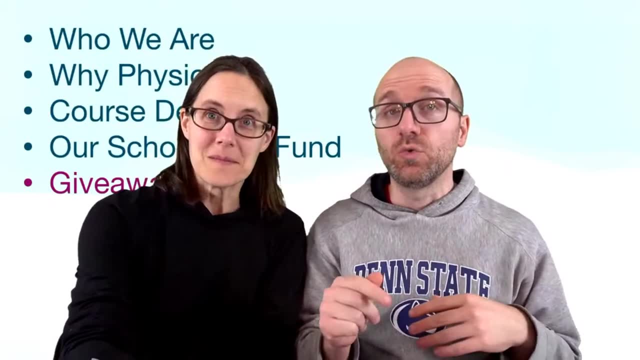 Eastern on Mondays and Wednesdays from September to December. That's right. So there'll be live sessions, Although if you miss the live sessions, I assume we'll have lots of families who just do the recorded sessions. Yes, And then great question from Emily that we'll answer before we do our giveaway. 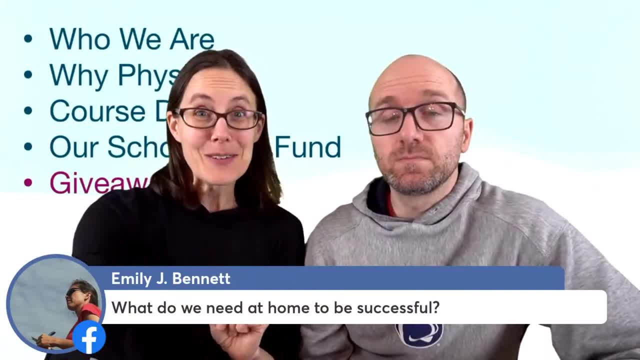 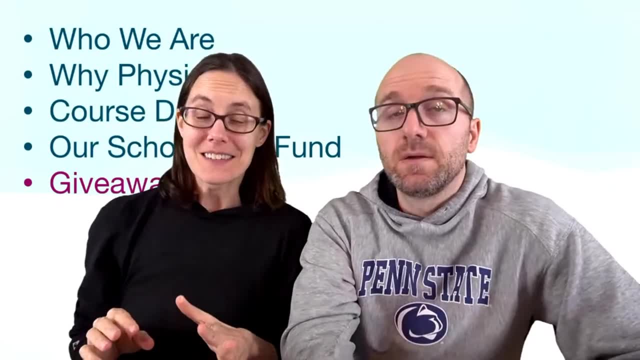 What do we need at home to be successful? I have to tell you, deciding which experiments to include in this was, sorry, a little bit challenging because there are so many to choose from, But we really prioritized materials that were easy to find. 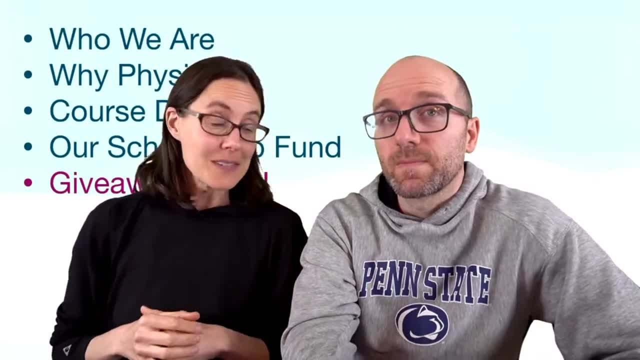 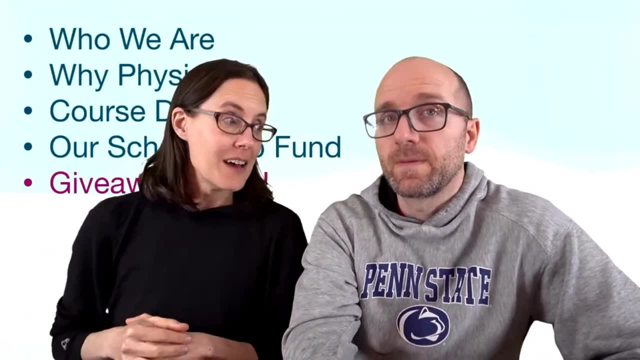 So for almost all of the experiments, except for the water rockets, we said: OK, we want to keep it to materials you either already have at home or you can easily find at the grocery store or a craft store, And you can. you can see a supply list. 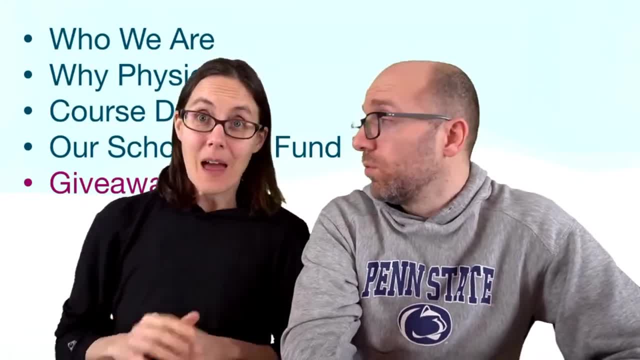 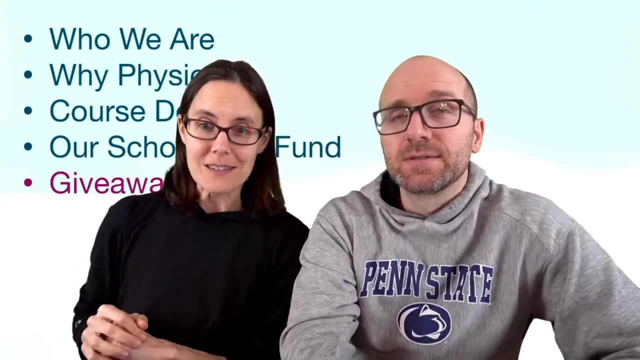 in the in the notes. That's right, And we will be doing supply boxes, but we don't have them ready yet because we're still kind of figuring out price and getting quotes from for a few different things. That's right, We're headed to Alaska for the summer. 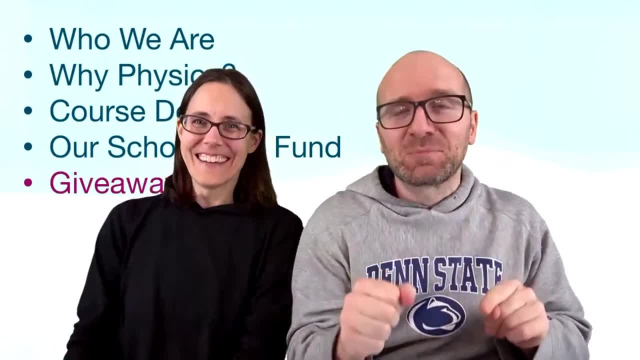 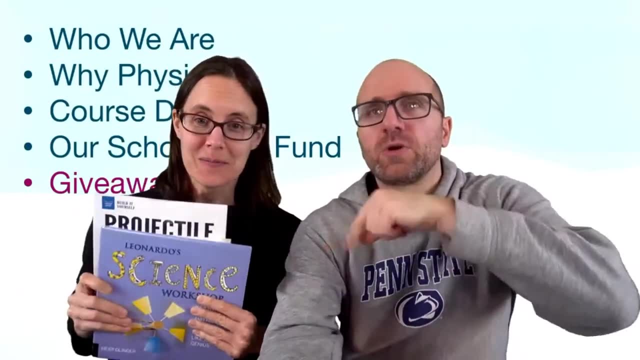 And there's some complications in the logistics of the supply boxes, But one way or another we will figure it out All right. So for these three books and one of the book titles, again book titles, again: projectile science. We're giving this one away twice, both in our teacher bundle and in our student. 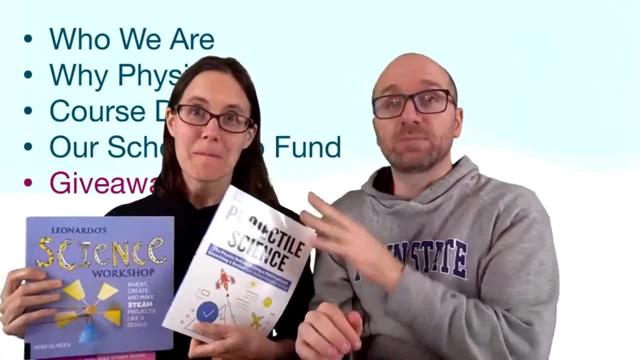 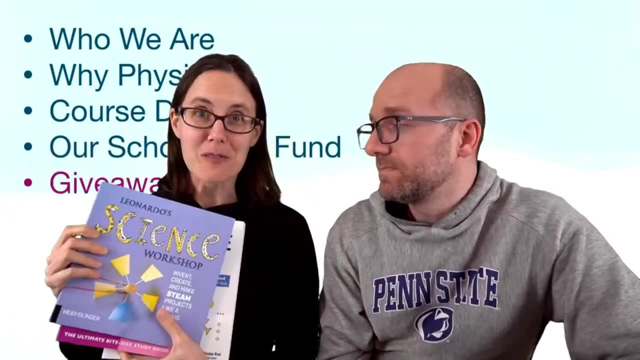 bundle, because we like it so much And it's definitely the one that fits this particular semester's topic the best. Yes, And we also have Leonardo's science workshop. I really just liked that this one had a bit of a history and a story aspect to it, as well as lots, as well as lots of fun. 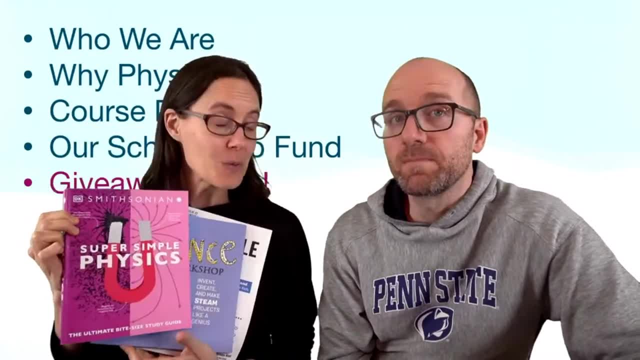 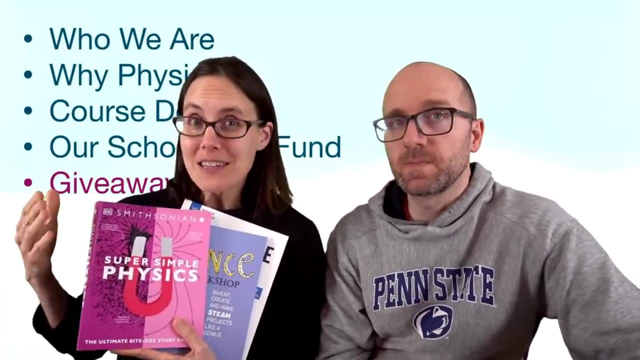 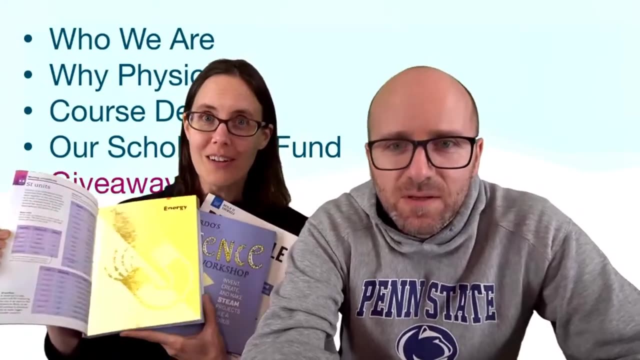 experiments and then super simple physics. This one's not so much an experiment book as it is just a theory of physics books, But it covers everything from energy to sound, to light, to mechanics, And it has a really beautiful illustration And graphics as well, which the green screen just doesn't know what to do with. 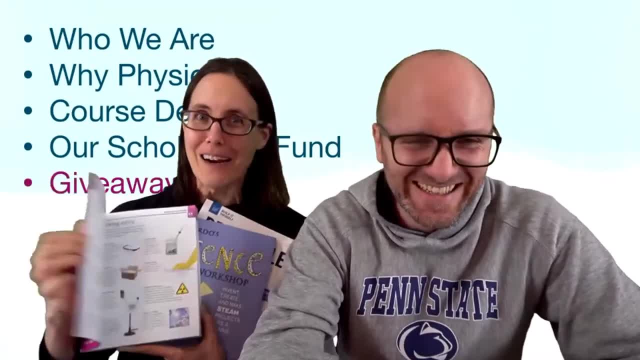 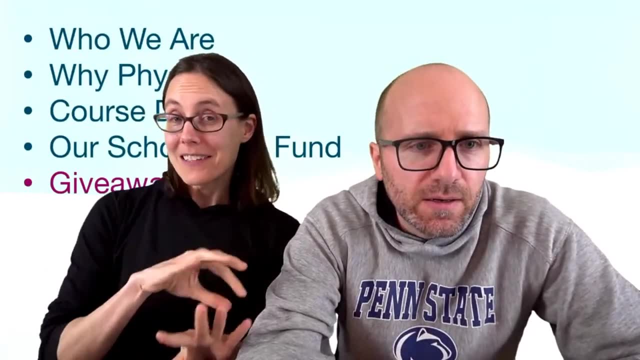 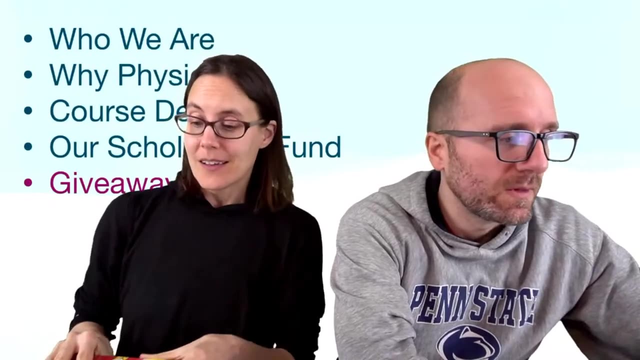 It's like the color green: It's everywhere, It's everywhere. All right, I'm opening up the spreadsheet right now. So what we're going to do while Math Dad is opening it up and getting it ready, we are going to draw two random numbers for our giveaway and we will give away our 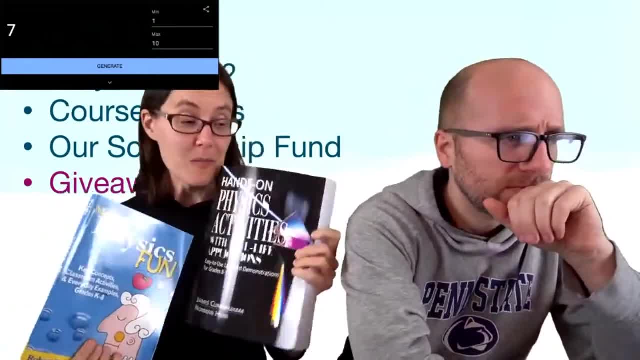 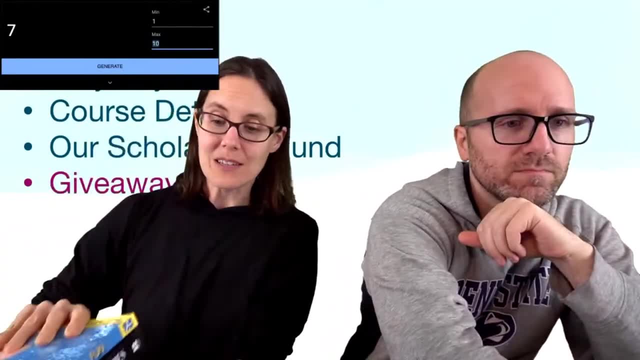 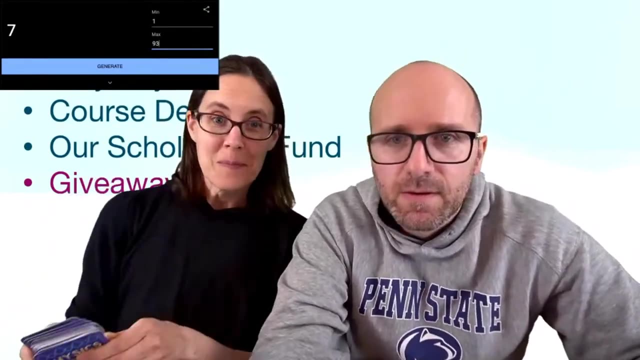 book bundle number one, our book bundle number two, which has more substantial, You know, if you're more designed for a teacher. And then we are also going to give away the several sets of these physics cards that I made. And oh, I have pictures of the physics cards: Math Dad. 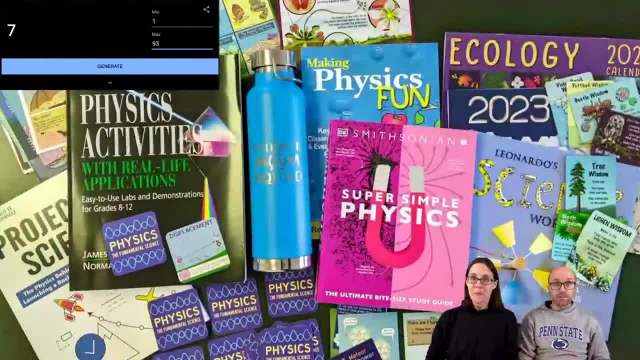 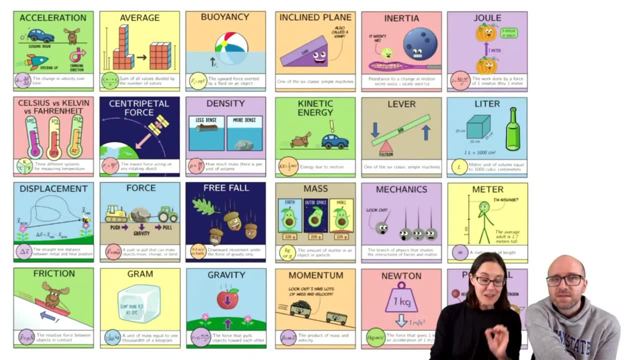 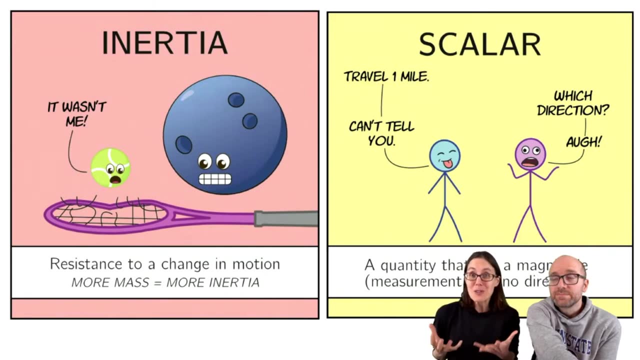 Really fast. OK, I made little cartoon cards, physics vocabulary cards. This is part of our physics course- that you can print out and then play the game memory. I really had so much fun. I'm doing this because you know, a lot of physics is just learning the language, learning the vocabulary. 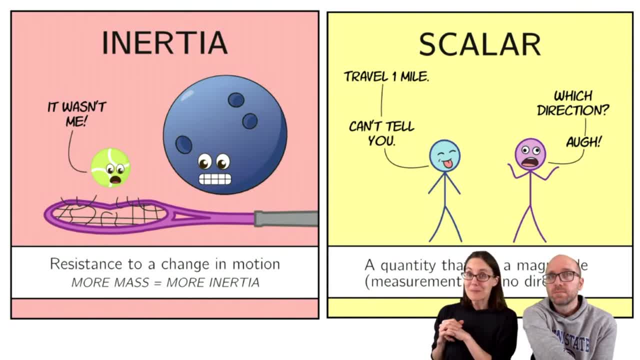 So here we have an inertia card where the little tennis racket is like. it wasn't me, because the more math something has, the more inertia, as the more resistance it is to a change in motion. And then scalars versus vectors. We've got fun little comics in the cards and I printed them so that we can have. 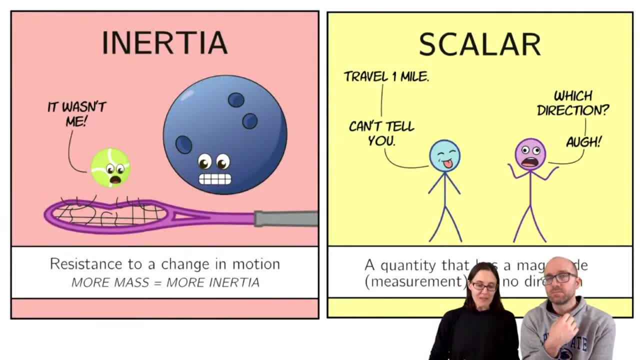 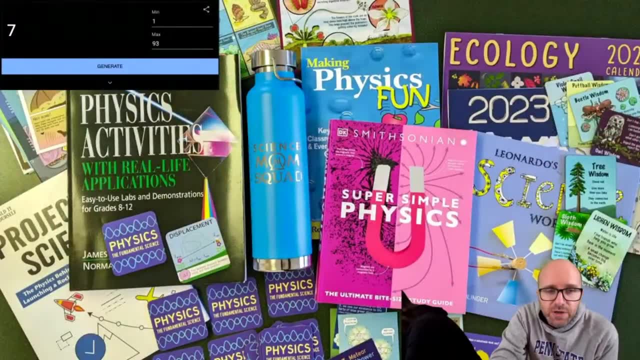 like a full on memory game, and we will be mailing those out as well. All right, Now I think we are ready for our giveaway, Math Dad. All right, So I've got my random number generator there. We currently have, say, ninety five people in the survey. 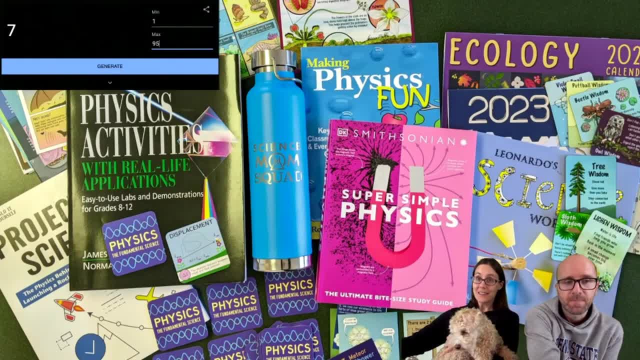 So we're giving away what with this first one. The first one is the physics books for middle school students, plus a water bottle, plus the memory game, plus as many fun things as we can fit in a flat rate box. All right, The first winner is: 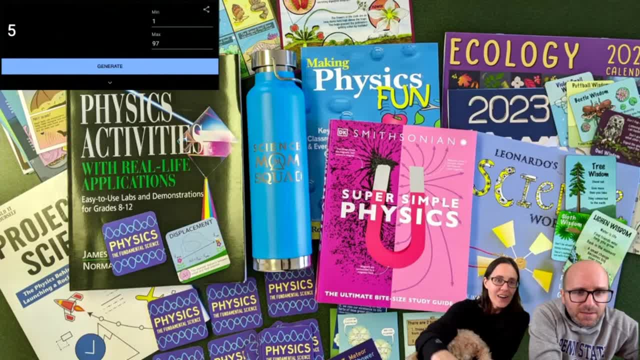 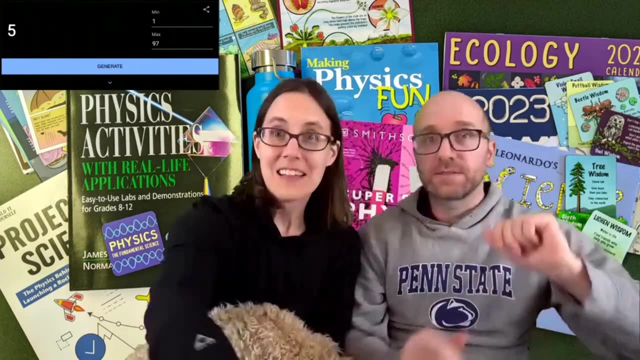 Number five. number five is: Oh Ken and Carolyn Owen in California. I get so excited when it's a name that I recognize: Yay, Excellent, Congratulations. All right, That's our first winner. Yes, What do we have up next? 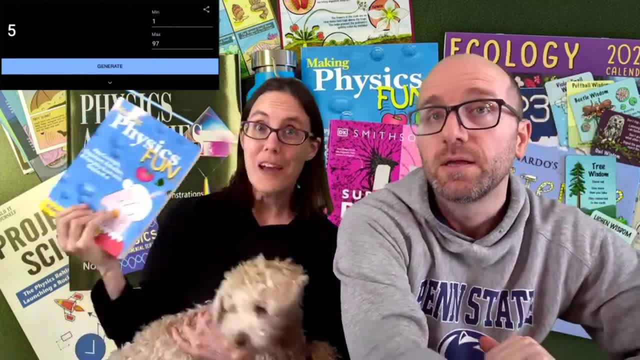 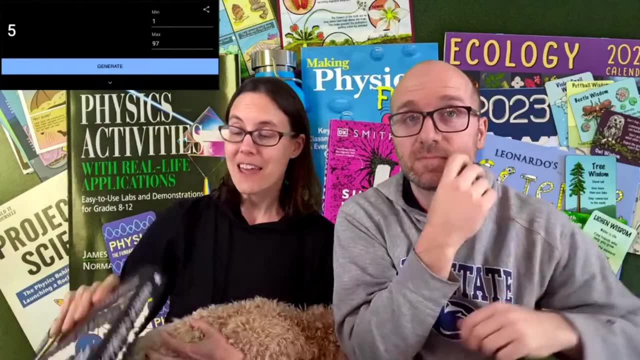 Next we have our teacher books. So we have making physics fun, which has fabulous, really fun activities for all sorts of different topics. And then we have hands on physics. This one's a little bit more robust, kind of designed for like high school. 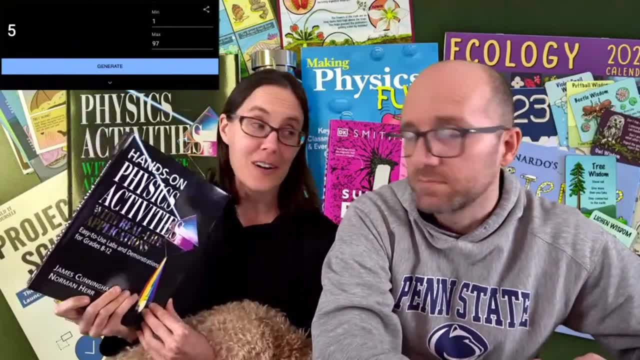 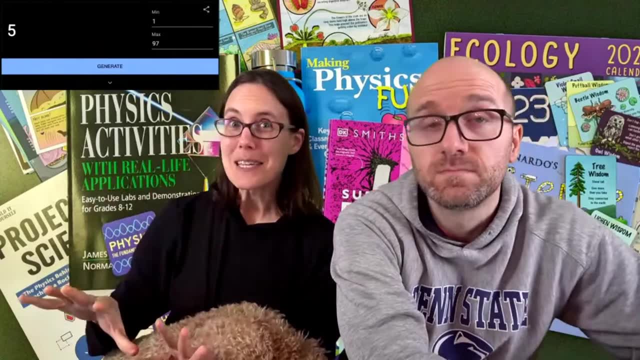 Um, but I love how detailed the explanations are. So it's got explanations and kind of practice problems and questions. So you do an activity and then it will really take you deep into exactly why and how the activity works. And we also have projectile science. 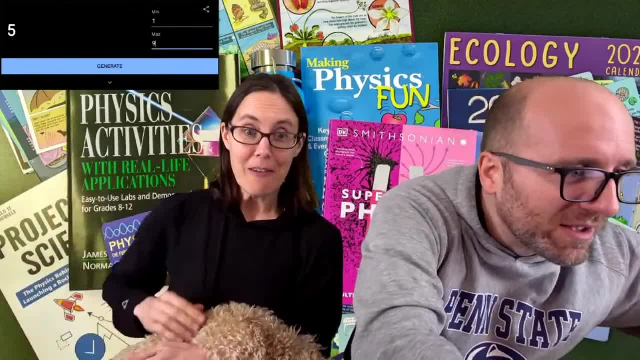 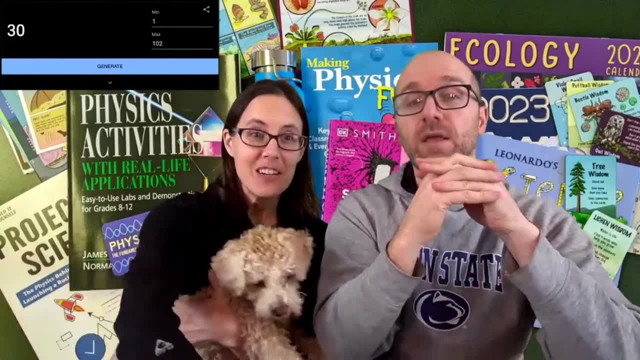 So those are the three books in our next bundle. We now have one hundred and two entries, So Math Dad's got to pick a number between one and one hundred and two. All right, The next winner is number thirty, Number thirty. I got to scroll up. 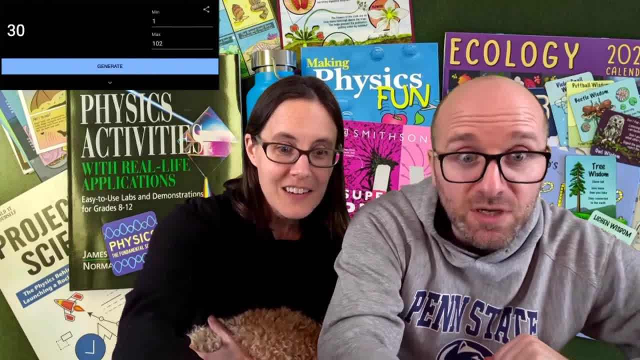 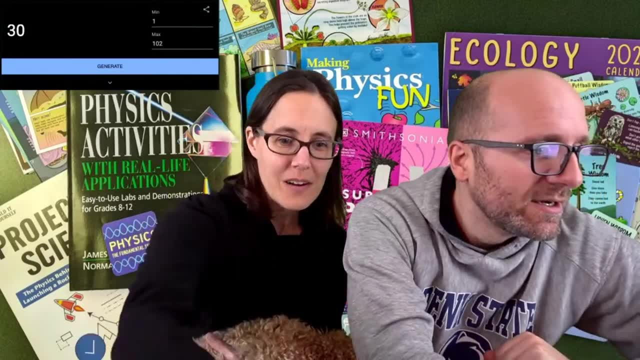 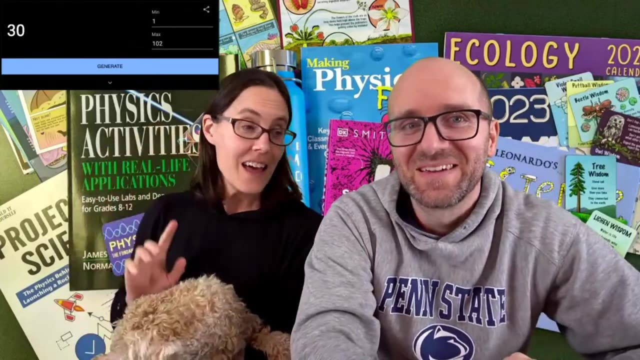 He is Kelly. Look, look what are Kelly. Look what are a. congratulations, Excellent. We are going to send you a big box with books and all sorts of other goodies like what you see here behind us. And now for the next part. 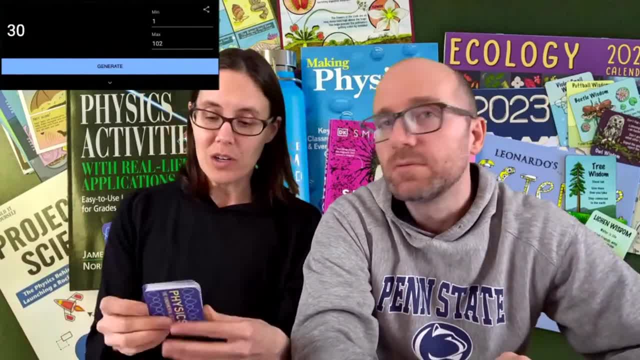 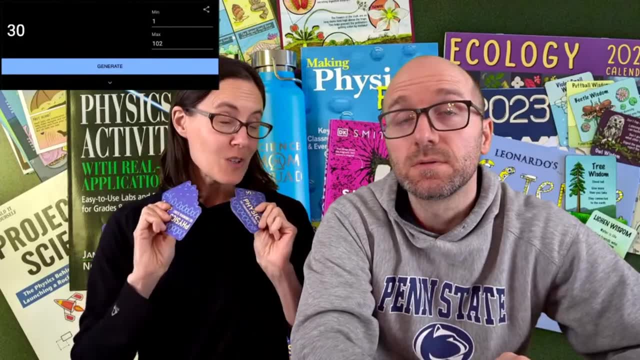 So we're going to give away. You know we're going to do it. We're going to do ten of these sets, but instead of doing ten numbers and having to scroll through our sheet, I think we should pick one number and then we'll. 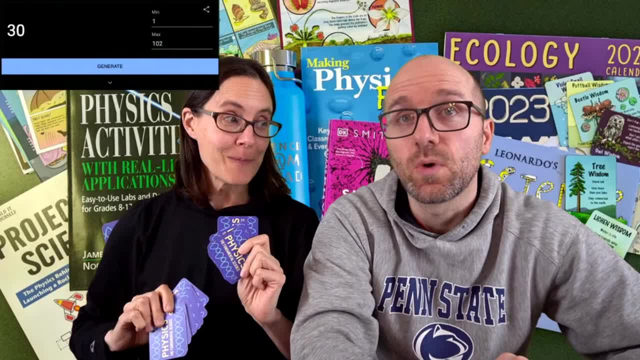 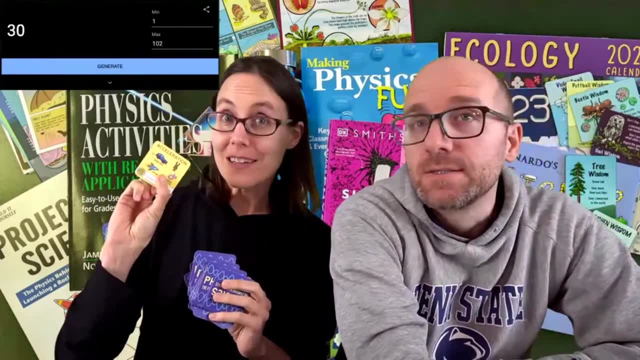 just count down ten names, You ready. What do you think? Math Dad, Oh wow, That's madness. But OK, no, that's, that's random. So ten winners are going to get a printed set of our awesome little physics memory game with all of the cards. 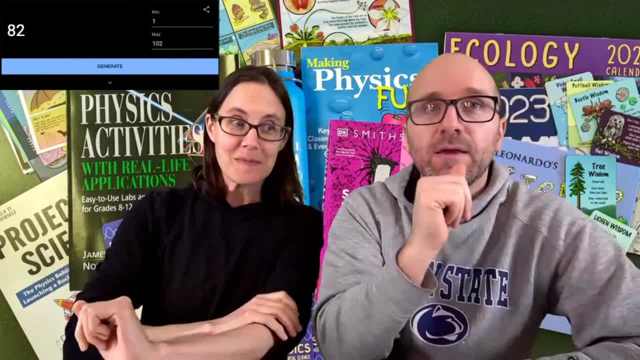 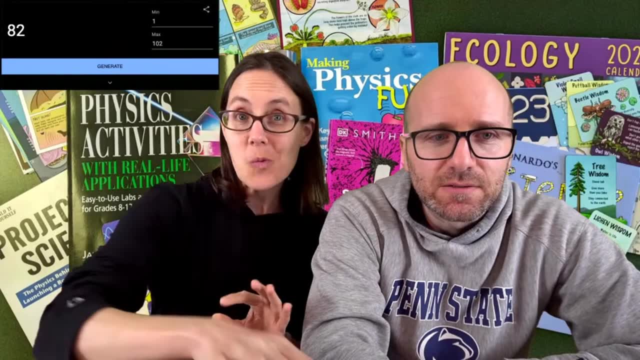 All right, Are you ready? And Number eighty two: All right, So get ready for a whole bunch of names, And we are going to email everybody who won a prize tonight, And then we'll also send you an email with a shipping number when we ship them. 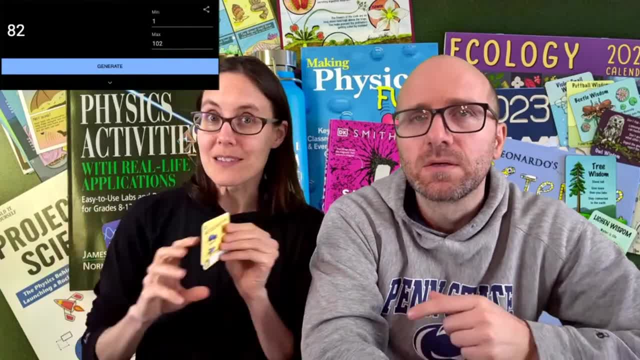 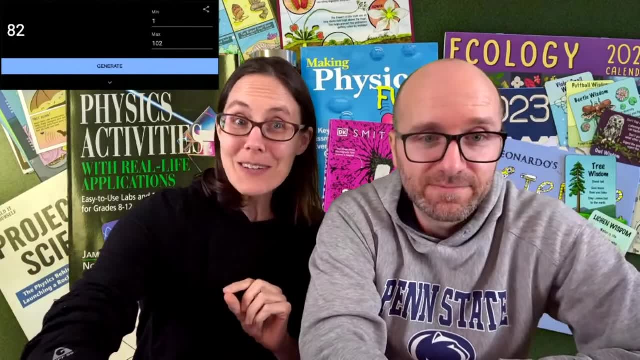 It'll be like probably this Thursday or Friday, because we're still waiting for these to get finished with the printing, Or longer. We will email you when we ship them. All right, We have Pam Stallings. Congratulations, Pam Maylyn Rosario. 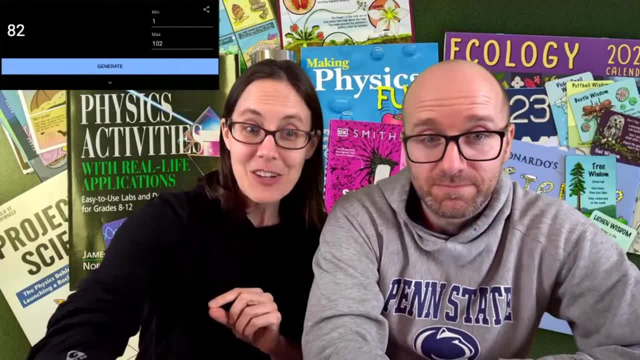 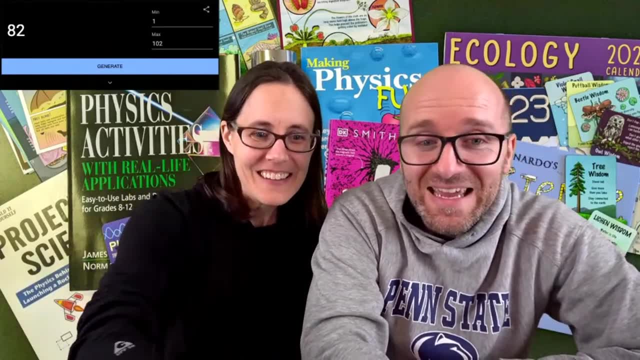 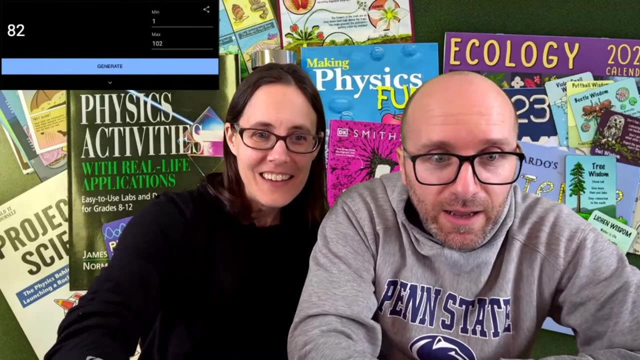 Congratulations Maylyn. Jelena Edwin. Congratulations Jelena. Maggie Iverson. Maggie Iverson. Congratulations Melissa Tardif. Manny S Congratulations Manny S. Noel Branda. Congratulations Noel. Adithya Mani. 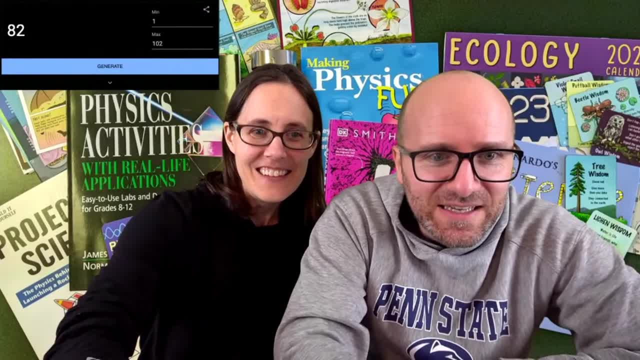 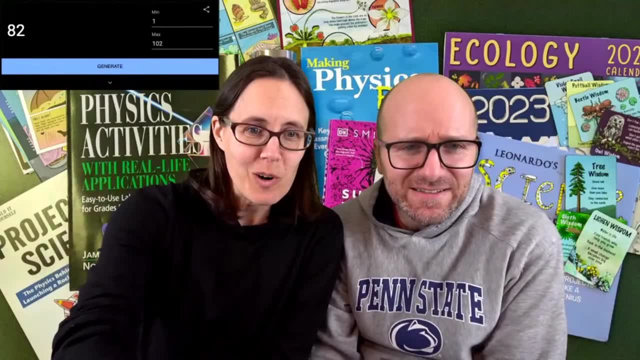 Adithya Mani, Carly C Anyan And Monica Platt. Congratulations, Monica Piet, And one, two, three, four, five, six, seven, eight, nine, ten, That's ten names. Congratulations to all our winners. 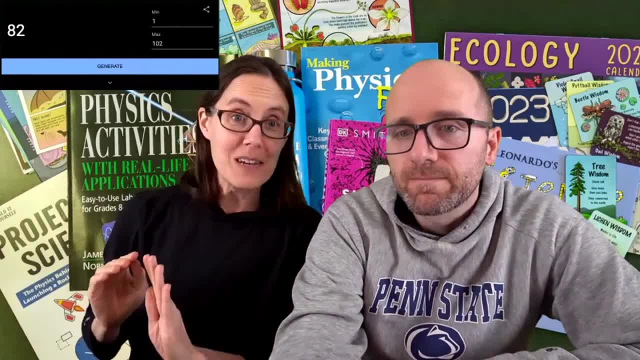 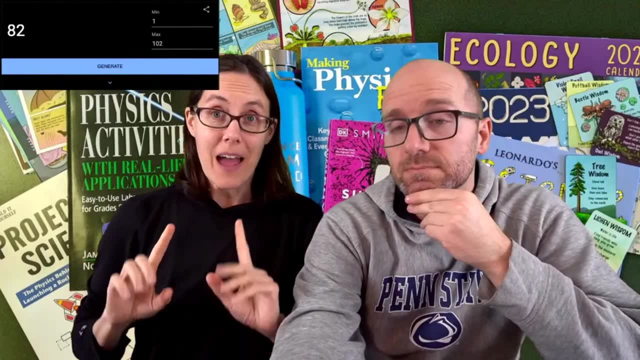 And now I want to come back and just take a couple minutes for questions and then we'll be done. So can the cards be purchased? They are going to be in our supply box. after we put them all in the supply box, If we have extras, I'll absolutely offer. 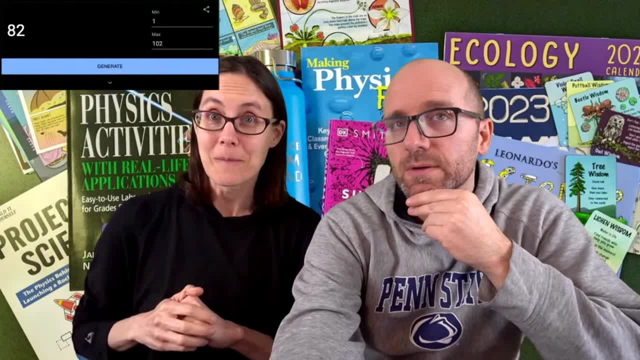 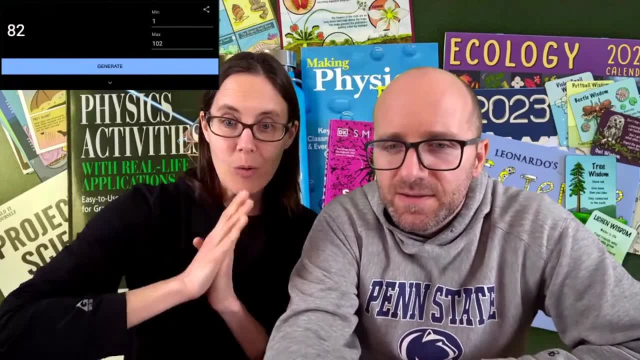 them for sale, but I'm not sure at the moment if we will have extras or not. That's right. So if you buy a supply box, then yes, you get the cards as part of it. Yes, And any other questions if you have any? 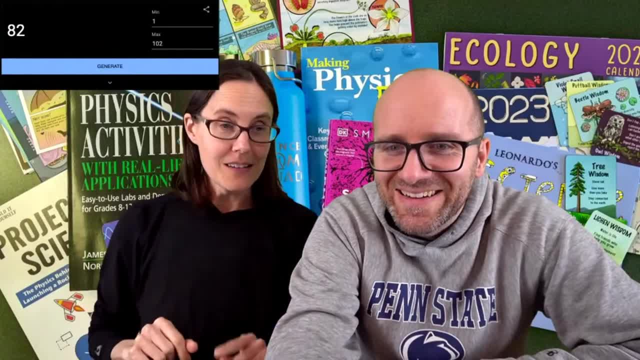 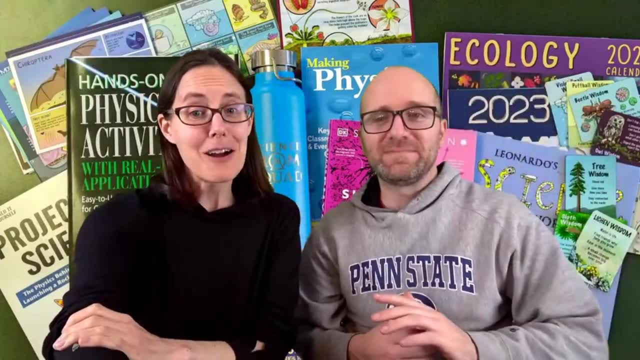 other questions about physics, put them in the chat really quick. And can we hide the black box? They don't want to see my random number generator. Oh, great Comment from Jelena. I struggled forever to find science that keeps my son engaged and he loves our. 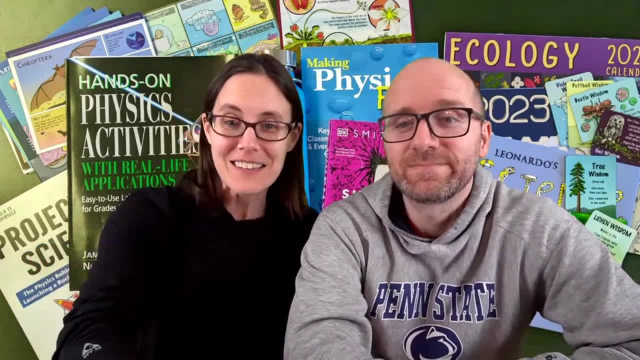 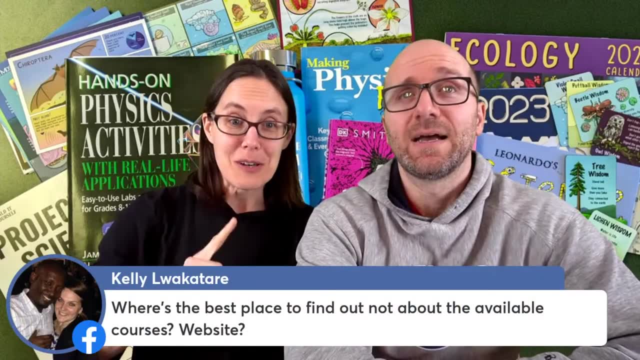 science class. I am so glad that really makes my day to hear feedback like that And and says: congrats everyone. How much does the supply box cost? We don't know yet. We will tell you when we know. Yeah well, where's the best place to find? 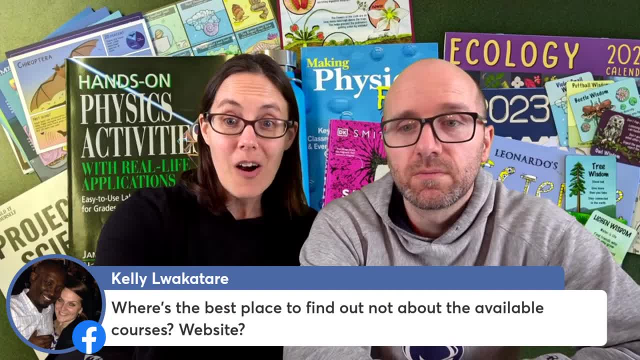 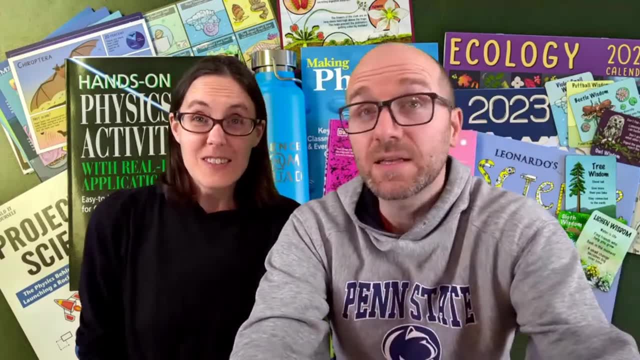 out about the available courses on our email list. We send send out emails and follow us on social media. Is that a good answer? That's certainly how to get the new ones, But if you just head to our page, I'll type it in. 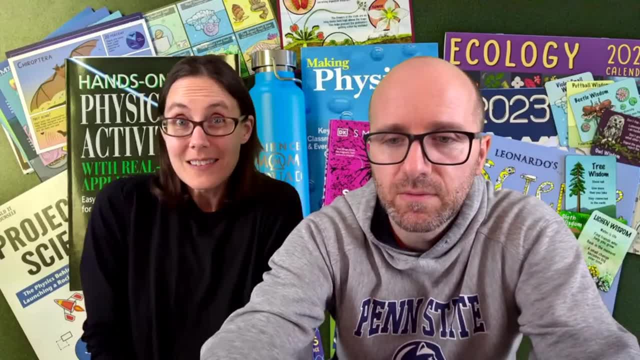 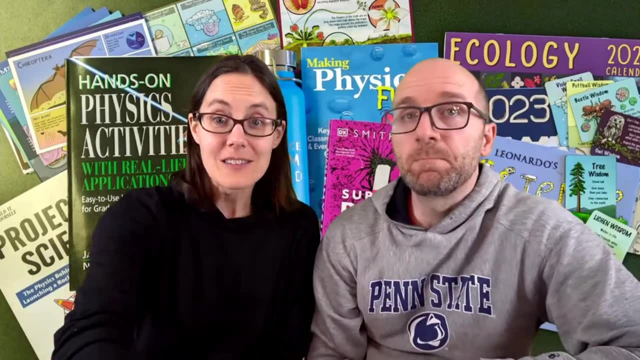 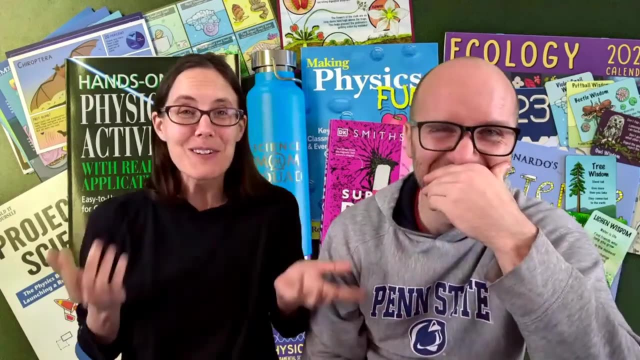 Science mom at teachable dot com or science dot mom. We have links to all of our courses there. The math that is putting that in the in the chat as well. Elena asks when will the supply boxes be available soon? No, Well, we will mail them out in August, but we'll. 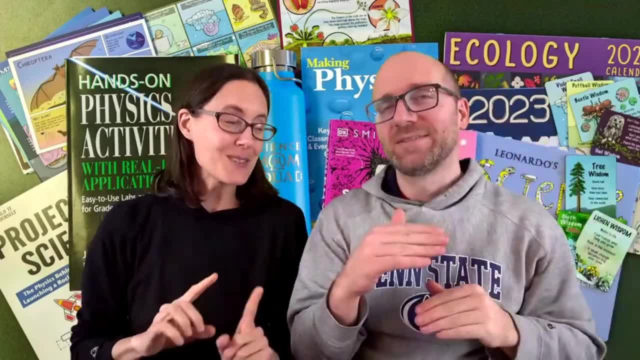 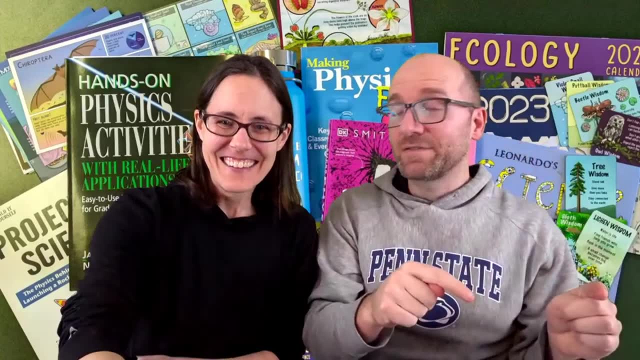 OK, you can order them, I hope within the next week or two. We're just figuring out. the ordering will definitely happen this spring, But delivery is probably going to have to happen after our Alaska, which means August is when they would ship out. 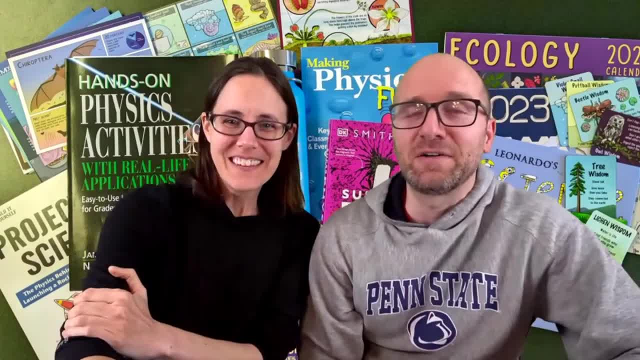 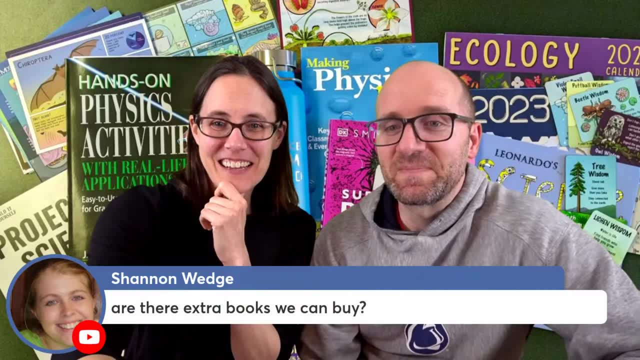 Yes, we would send them in August. That's the only way we think we can pull it off is get all the supplies over the summer, pack the boxes beginning of August, ship them off. And then Shannon asks: are there any extra books we can buy? 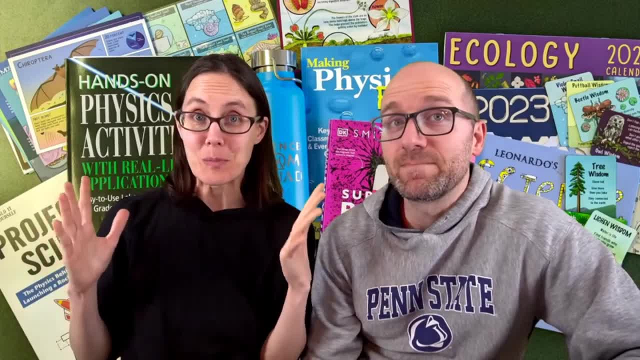 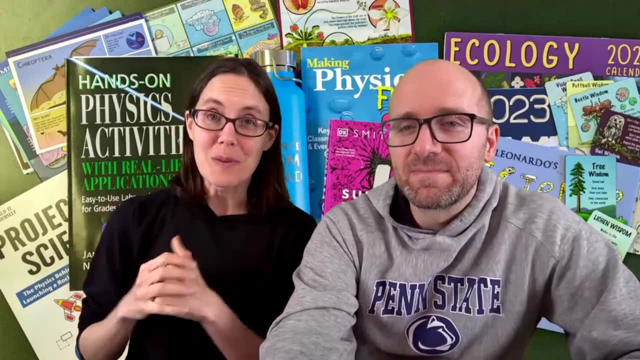 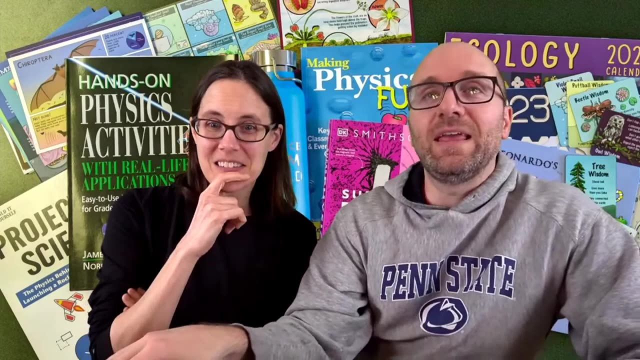 I. I have really enjoyed expanding our physics book library. as I've been researching and preparing this class, I will definitely, on the course Registration page I'll have a little bonus section where I'll just give some book reviews of my favorites. But but yeah, if, if. well, if one wanted one book, this is one of our. 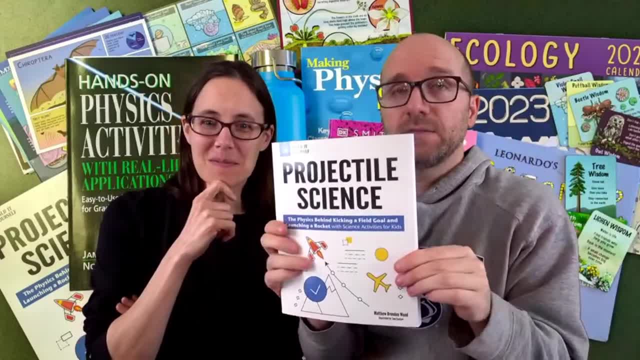 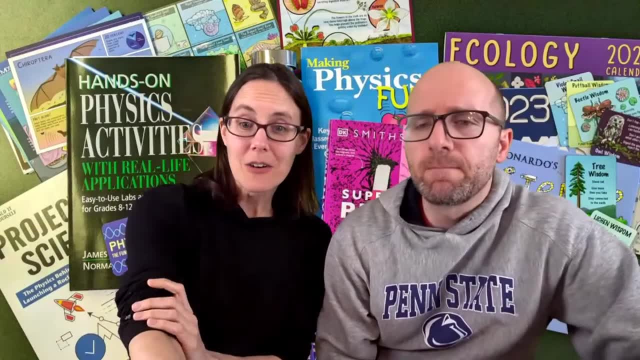 favorites, the course for this fall, the absolute best projectile science. Yeah, we'll be hitting just about everything in here and in one form or another. Emily has a great question about labs, our labs, all done on one day of the week. 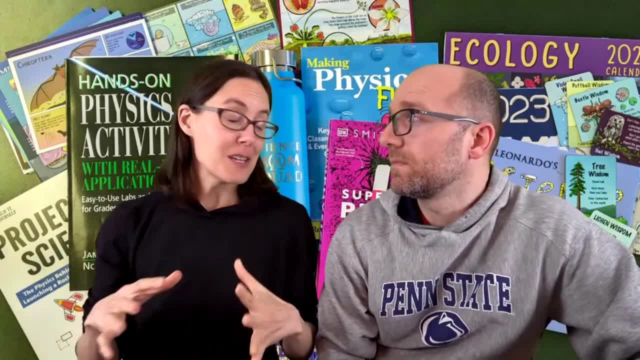 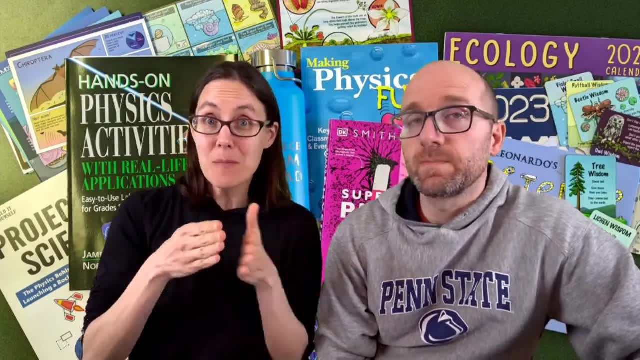 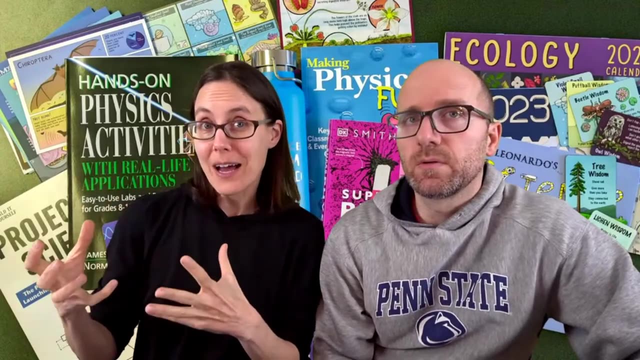 So the way we have it set up is that the labs or the hands on activity portion, those are all self paced videos. So we have the Monday and the Wednesday live lessons and then any time between Wednesday and the next Monday there's a self paced video lesson with the hands on activity or the lab. 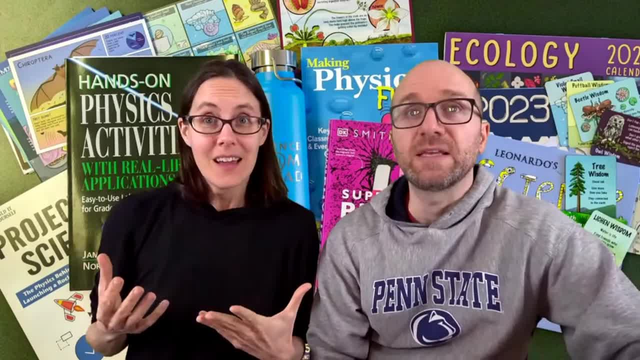 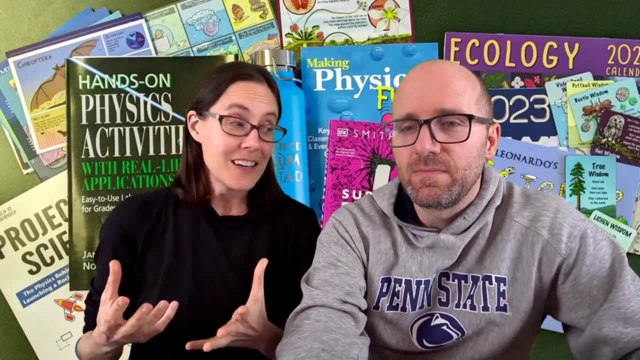 Yep, So some project to do? Yeah, your own pace And you can really be flexible with those. It's ideal if you can do them in sequence, But if you don't have materials for one and you need to like substitute or switch around the order, that's totally all right. 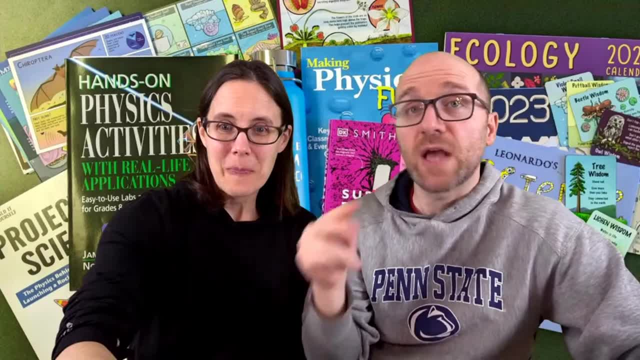 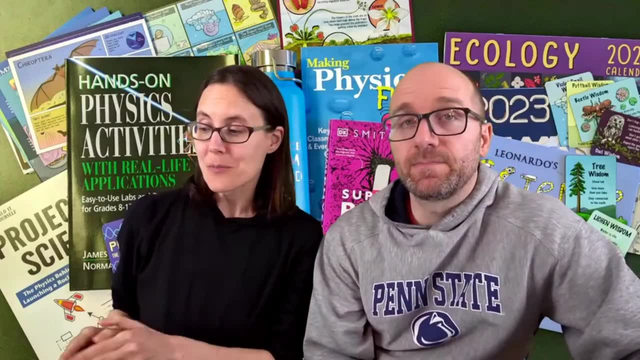 That's right. So the live lessons Monday and Wednesday and you can choose either session to attend. And then there's the third lab or project. Yeah, And then Michelle asked: do we have a book list somewhere? The links to these books I will put in that I mentioned I will put in the description. 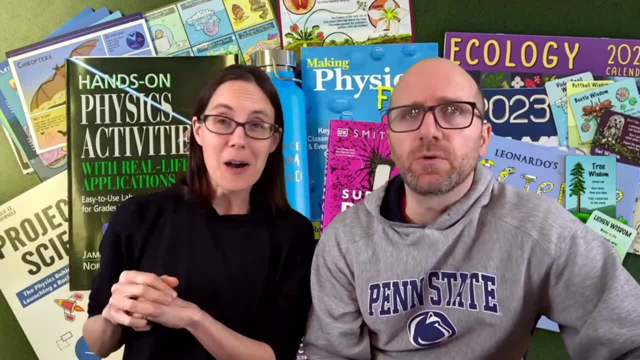 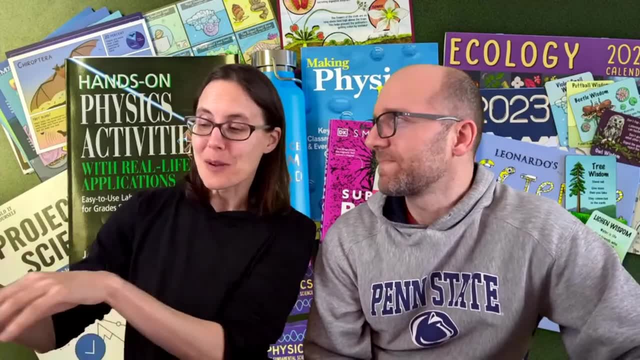 of the video so you can find that on YouTube if you're watching later. Although clearly we need to add it to, I am going to be building a more robust because you know this is sort of narrow, like for teachers- my favorite- and for middle school students. 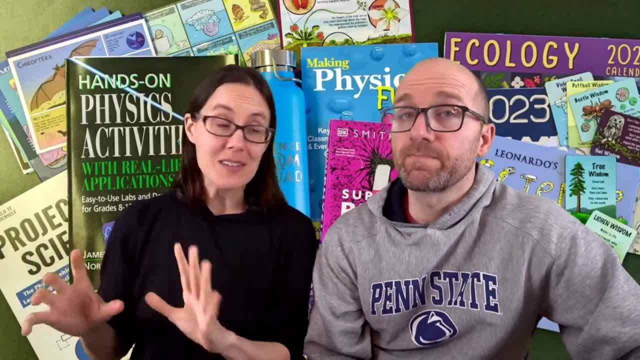 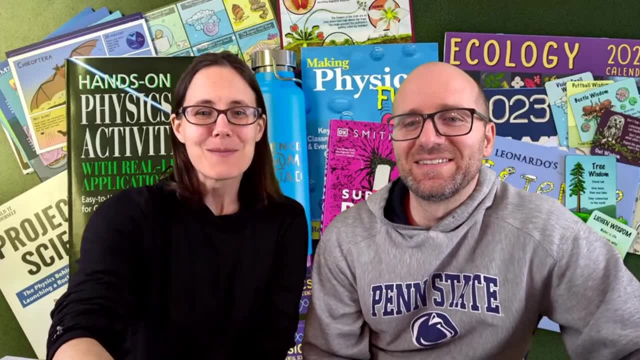 But also we found some really great books for my students and I would like to build more of a robust book review like blog post or something. Elizabeth has a fabulous question: What's more important- physics or chemistry? Dun dun, dun dun. 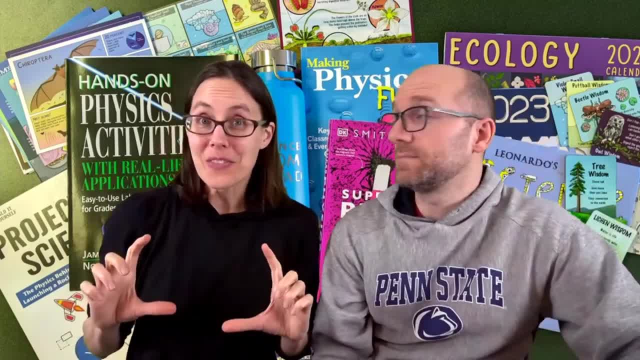 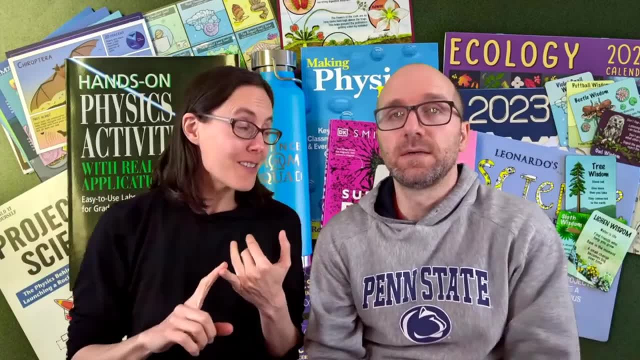 Physics kind of has the right to claim that it's the foundational science and that it is every other type of science. really, It's like it has tons of math and it goes from like quantum, like the smallest realm, and and includes some chemistry in it. 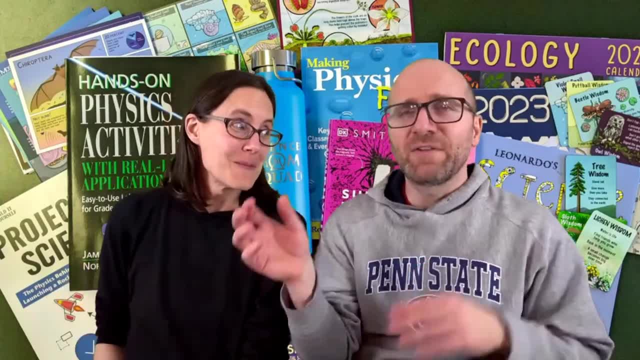 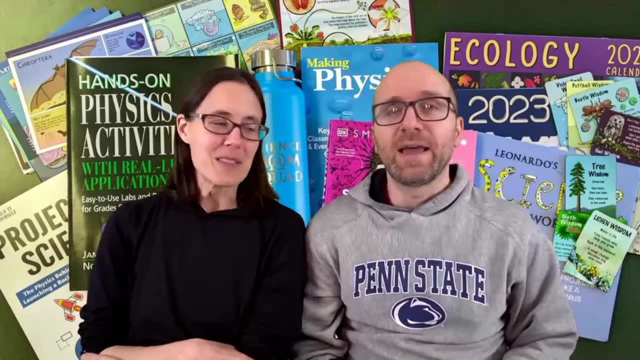 And it's like well, it intersects all of the other branches of science. Pretty much every other branch of science was at one point part of physics and it got too big and it just kind of like butted off to its own thing. Yeah. 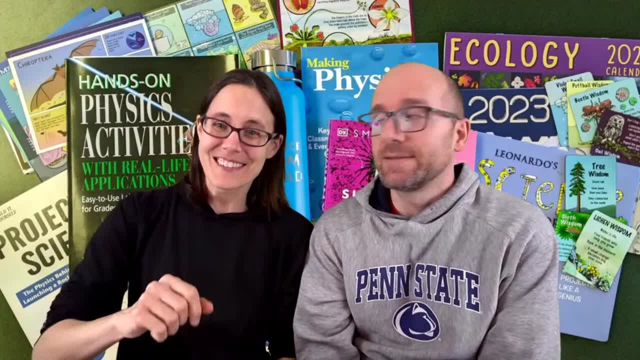 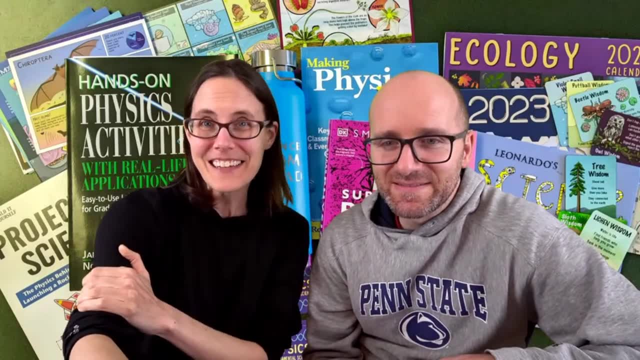 But then physics was like I will stay the biggest and the broadest, because it still is one of the broadest sciences. That is a fun question. Oh, hello to Esther watching in Italy where it is much later than 9 pm. 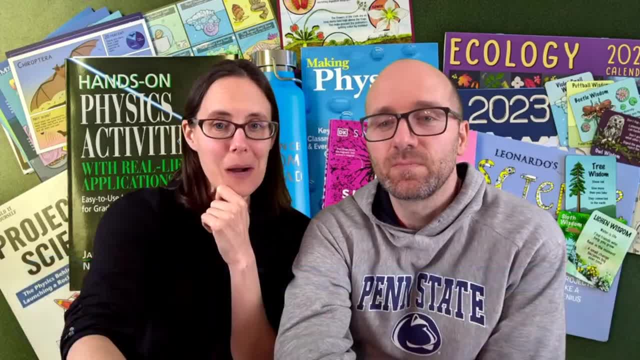 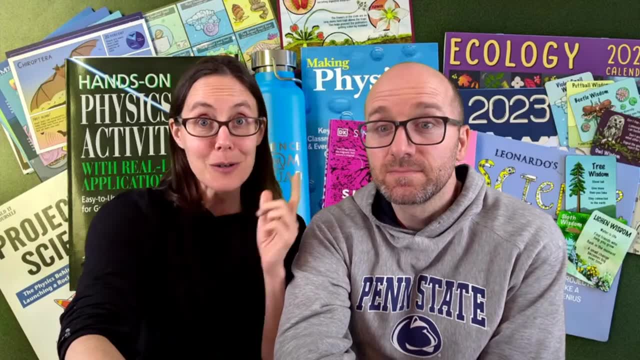 Oh, Kelly says would love to hear for about elementary age books too. I will write a bigger one. I will write a bigger blog post. Any other questions, type them in real quick. But it is late at night for us and also late at night for Esther watching in Italy. 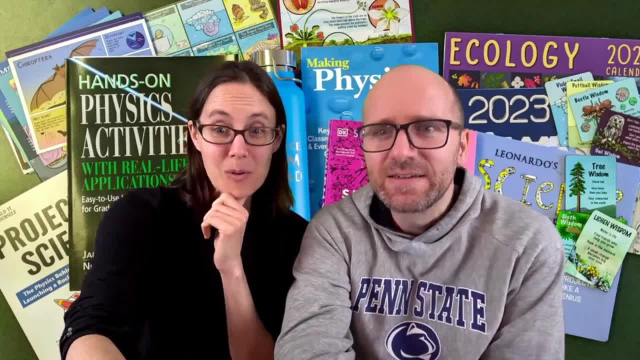 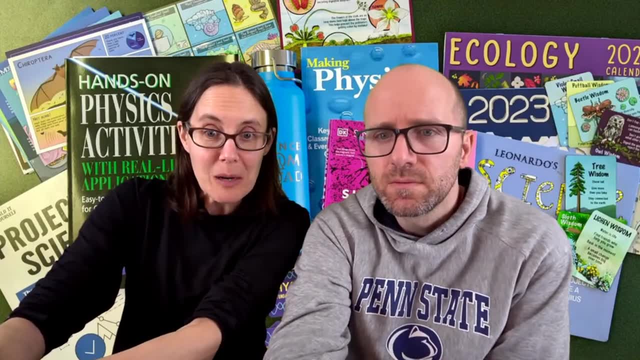 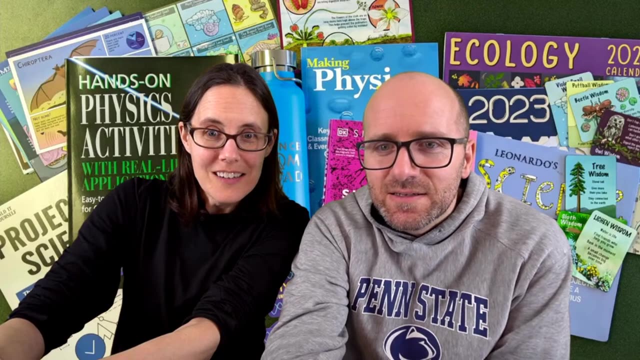 So we are going to wrap it up pretty soon. I did see a couple of questions about another physics curriculum called KSP2.. I'm actually not familiar with it, but if you email me I can kind of look up to it And I think we- I think we- collected most of the questions.